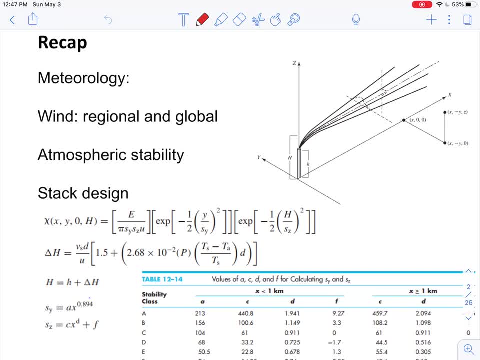 in the transport of the air pollutant And at the end of the class we introduced a stack design. So more specifically this is talking about the transport of air pollutants coming out of a stack. So I didn't got time to introduce the detailed procedures for solving these problems, So here 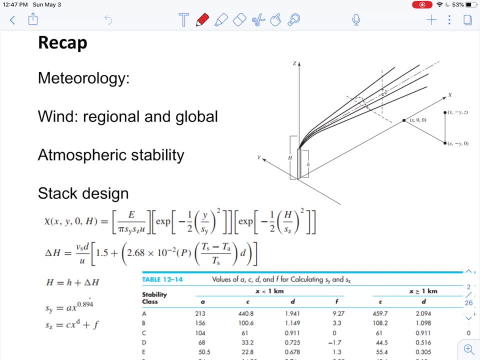 I'll just go through this procedures again, but without detailed numbers here. So basically, the, the system we're talking about, has a geometry. it looks like this: So we have a stack that has certain height- this is the real height of the stack- And then the air pollutants are going to get emitted from top of it. And then we designed 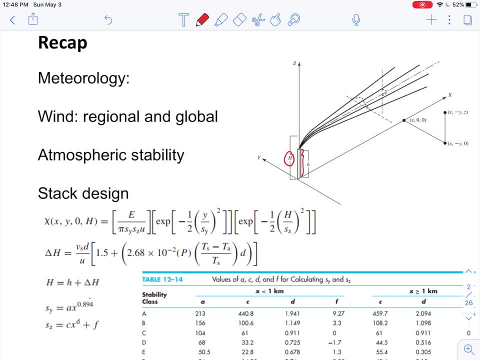 a parameter which is called the effective stack height. So, basically, the air pollutants will first travel upwards and then follow the wind direction, which is along the y direction, which is along the x direction. So that's why we designed a effective stack height for a stack, and then we can apply the air pollutant to the stack. 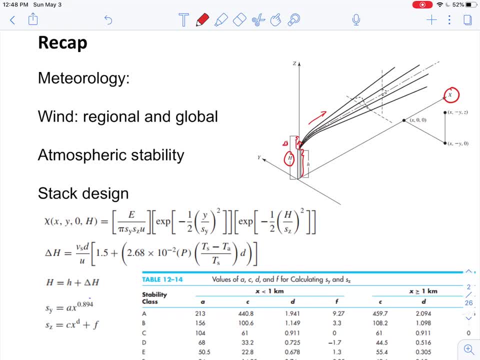 which is okay. So we have. so we have a stack that has certain height. this is the real height of the stack. stack height where we have to include the vertical transport at the beginning of the transport And then, as the air pollutants are further being transported, they're going to get expanded. 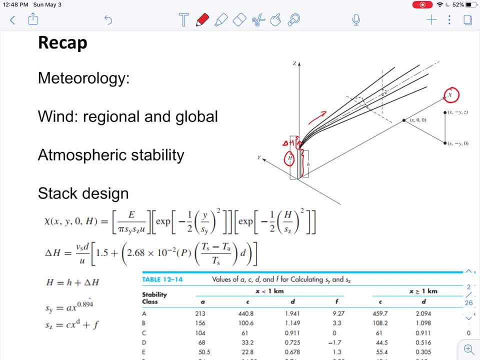 both in the y-direction and z-direction. So basically the transport will follow Gaussian distribution, where the concentration at the center is always the highest, while the concentration at the edge are lowest. So they're going to follow the Gaussian distribution along the y-direction and also. 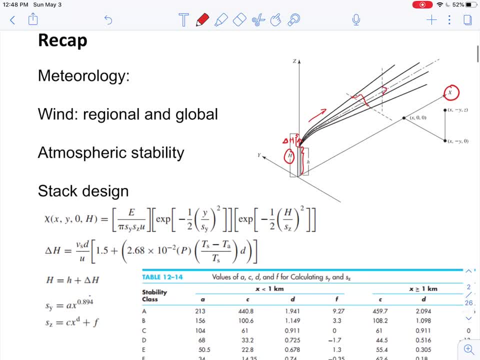 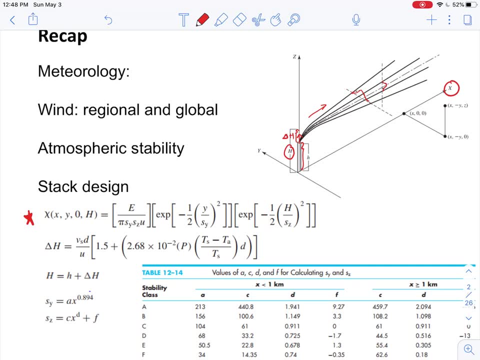 the Gaussian distribution along the z-direction. So what this equation tries to solve is basically: at any surface monitoring point, let's say we're interested in the air pollutant concentration which is 10 kilometers downwind the stack, and also out at the ground. 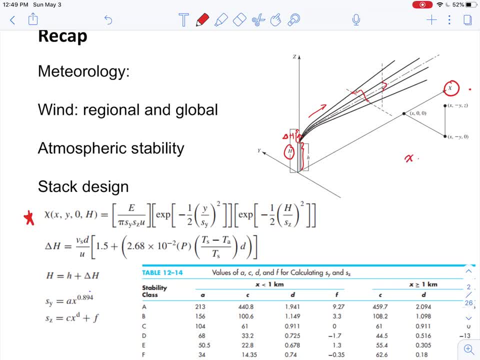 So what this means is that we have to know what is x, what is y, and here, since we're measuring at the ground, z is equal to zero, so we can basically try to look at what is the air pollutant concentration and any x, y, x and y coordinates. 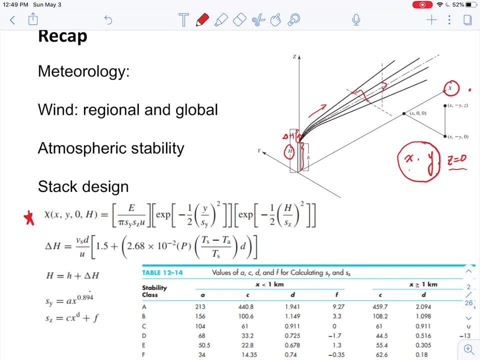 while the z equal to zero. okay. so, if we look at this equation, what are the inputs? we need to know what is x, we need to know what is y and also we need to know what is the height of the stack, which is the effective height of the stack, okay. so, for example, if you want to know 10 kilometers, 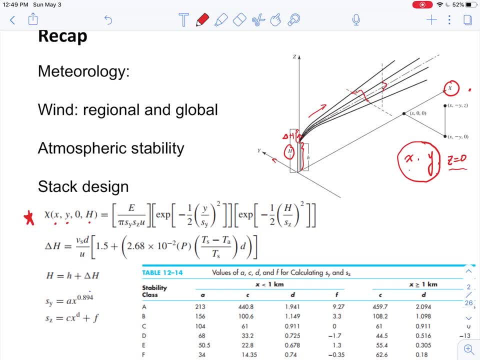 downwind, but also in the y direction, which is one kilometer away. then the x will be equal to 10. right y will be equal to one. all right, so basically we can use this equation to solve for the air pollutant concentration in there and also why we're interested in that is. 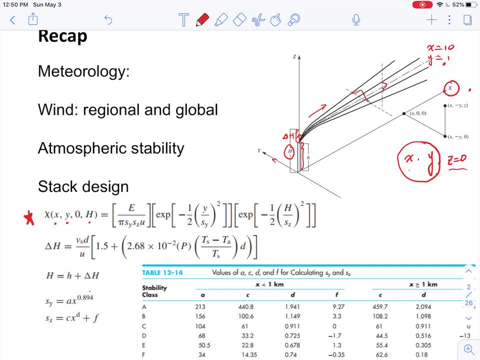 so if we set up a monitor, monitor, monitor and station at this specific location and then we can measure the concentration there, so we can use this equation to trace back what is the emission rate of the air pollutant which is the e value here. so basically you can see in this equation that we have several unknowns or 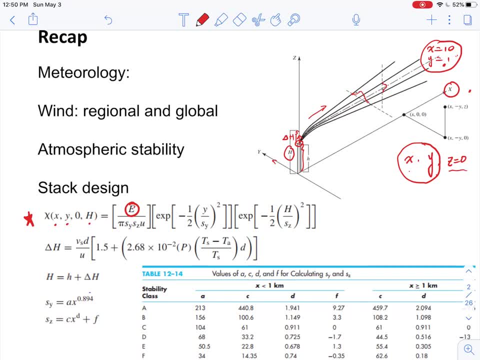 several parameters determining the concentrations at this specific s and y location. we have e, which is the emission rate- okay. and we have s, y and s z, which are the standard deviation of the spread of the air pollutant along the y direction and along the z direction. so remember, the dispersion happens in y and z direction, okay. and also we have 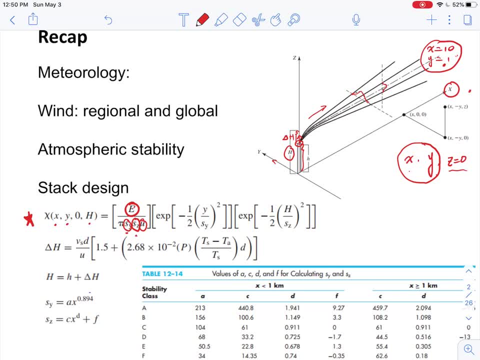 u? u is the wind direction along this downwind direction. basically, that's why the air pollutants will travel along this x direction. right, so this is just the wind um wind velocity. okay, so you see that once we have these three parameters here, um we can basically solve for what is the? 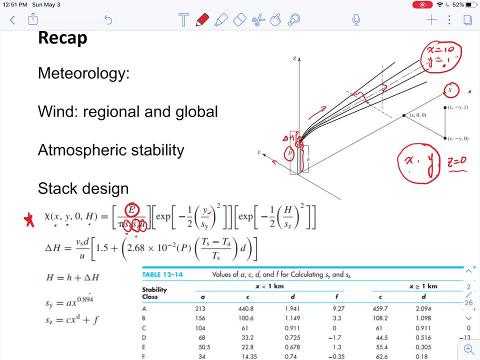 concentrations, right, we know what is x, what is y, we just plug them in, right, and then we should be able to solve for these uh concentrations at any specific location, right? so, um, so, by using this equation uh further, we need to calculate, um, basically, what is the emission rate of this air? 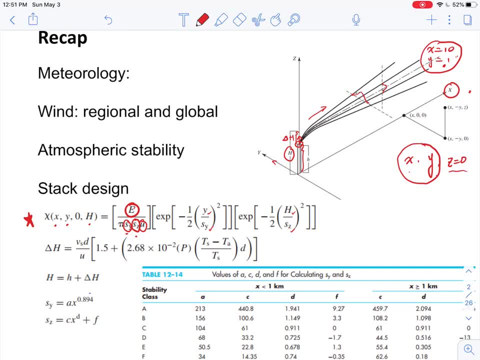 What is the h, which is the height of this system, the effective height of this stack? right, So the effective height can be calculated by summing up the actual height of the stack and this delta h, which is the additional height above the stack. 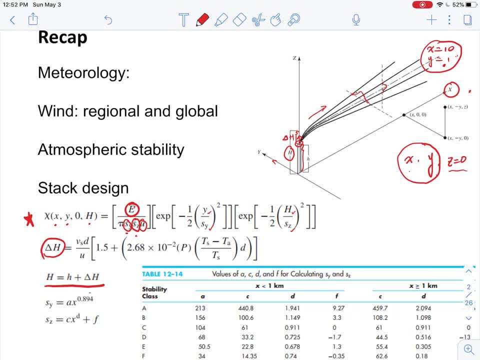 And we can use this equation. You can see that this additional height is related with what is the velocity at the outlet of the stack? right, Because the air pollutants are emitted with certain vertical velocity, which is Vs. okay, It's related with what is the diameter of the stack, what is the wind velocity, what is the temperature of the stack and temperature of the ambient. 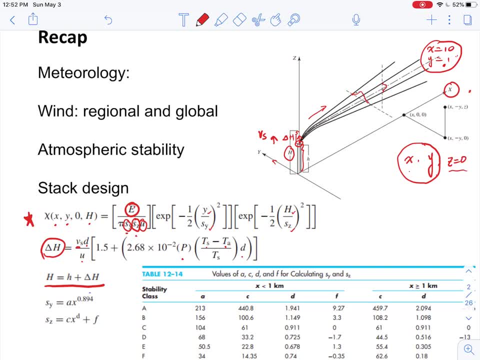 and the atmospheric pressure and also the diameter again. okay. So if we have all of these parameters, we can calculate h right, And then we know the wind direction. We just need to know what is the standard deviation along the x-axis. 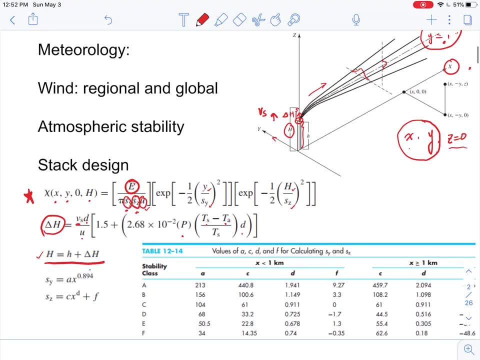 Along the y and z direction. So we mentioned that this is related with the atmospheric stability condition. So typically the problem will tell you whether it's during daytime or nighttime. what is the cloud condition, right? So basically you can refer to this table here to calculate or to trace what is the values of a, c, f and d right? 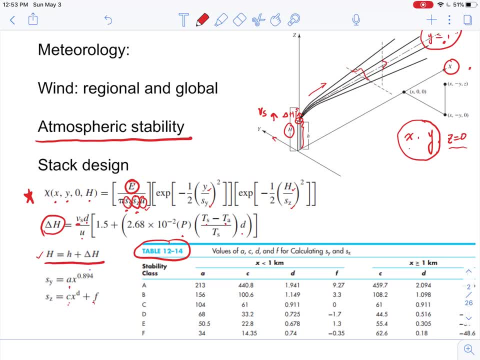 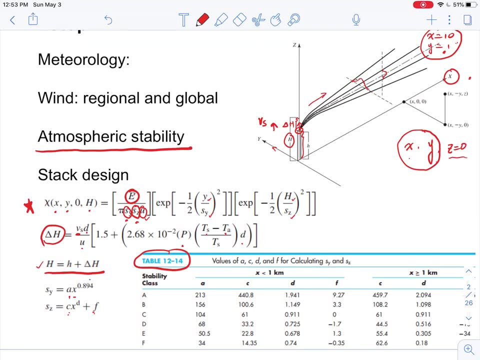 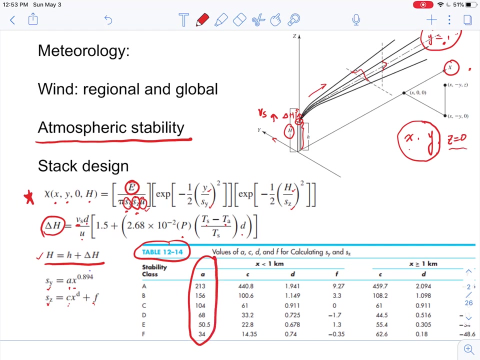 So basically you can plug in these parameters, Plug in the f, Plug in the x value, which is the distance downwind of this stack, right, So you can calculate what is sy and what is sz. okay, So again, you should notice that actually there should be a typo in this table, because the a here is not dependent on the x. 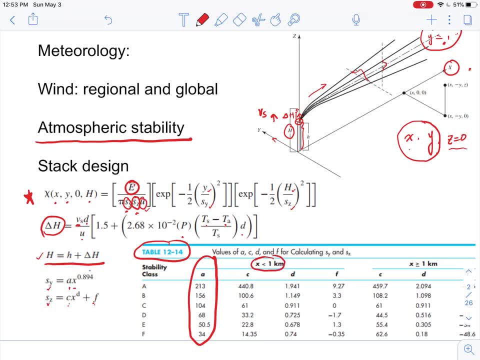 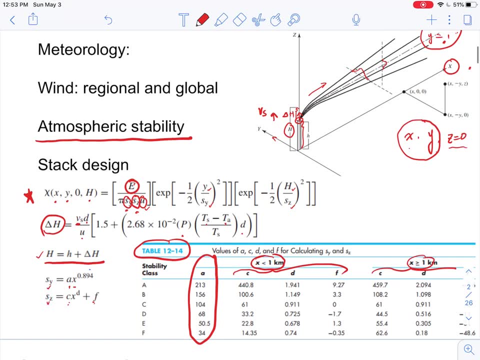 It's not dependent on the x value. So, basically, if the x is smaller than 1 kilometer, you can calculate that based on cdf. If x is larger than 1, 1 kilometer, you can calculate that based on these cdf values. 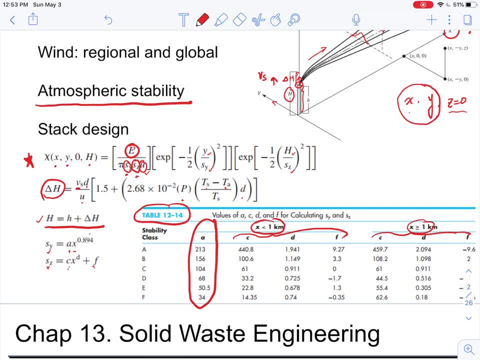 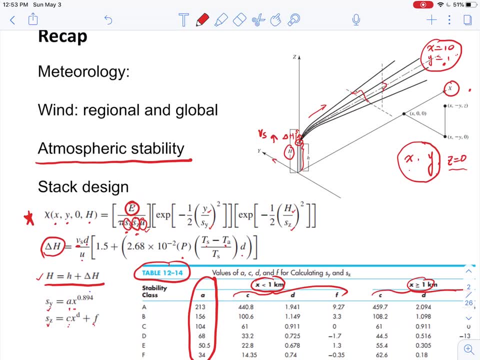 A is always the same. okay, So you can calculate the standard deviation. Now you can plug in everything to calculate what is the concentration at any specific location downwind of this stack And also if you know these concentrations, if you know the concentration, you can trace back to calculate what is the emission rate coming out of the stack. okay, 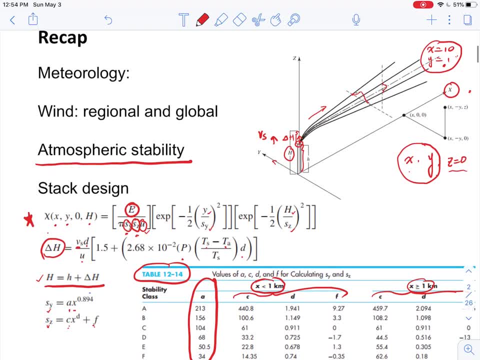 So I don't have any numbers. I'm just going to plug in this calculation process. but by working on the homework problems and also the example problem in the textbook, you can get more of a feeling in terms of how we can use these equations to evaluate the air pollutants emitted coming out of a stack. okay, 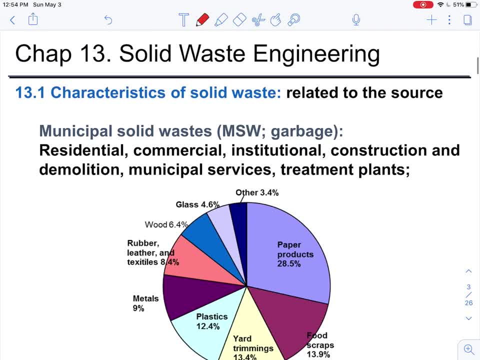 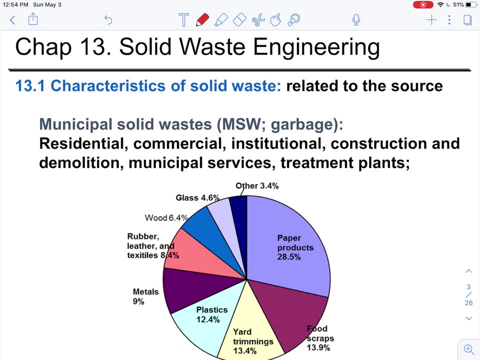 So, since we're getting into the final week of our 2601 class, we have to finish up on the final transformation. We have to finish up on the final transformation. okay, So until now, we talked about the water treatment, We talked about the wastewater treatment. air pollutants. 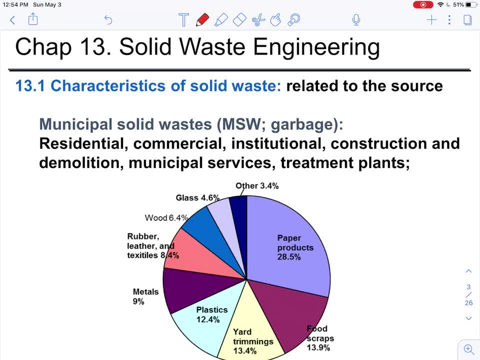 And then we mentioned that the pollution can happen in all different phase of the objects. right, We talk about liquid phase, which is the water and wastewater processing. right, We talk about the gas phase, which is air pollutant. So the only phase that's left is a solid waste. okay, 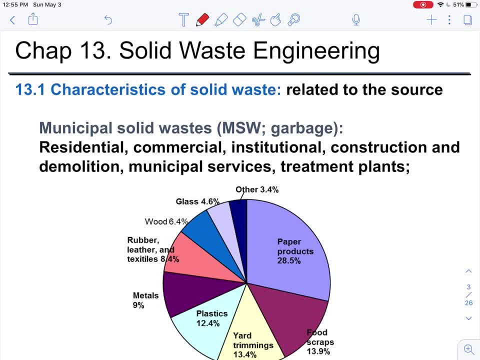 So, starting from chapter 13,, we're going to talk about the air pollutants. So, starting from chapter 13,, we're going to talk about the air pollutants. We're going to talk about the solid waste engineering and hazardous waste engineering. okay, 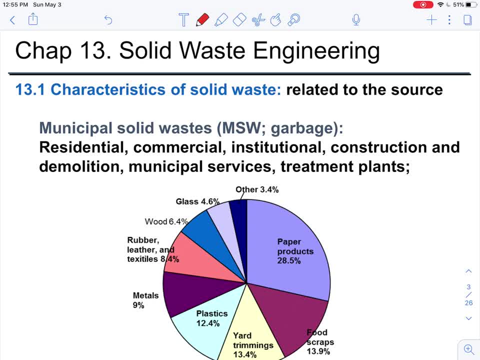 So typically these are existing in solid phases. okay, So we mentioned about solid waste. Actually, we generate a lot of solid waste by everyday life And especially right now, during the COVID-19 situation, we probably generate more solid waste because we're eating, making our meals at home, right. 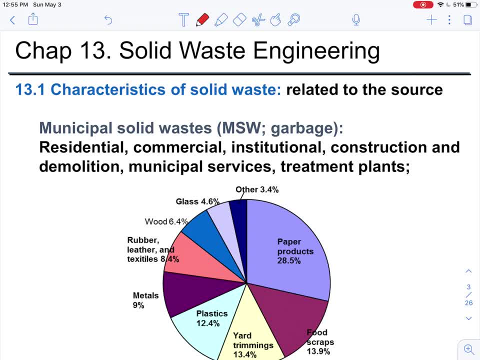 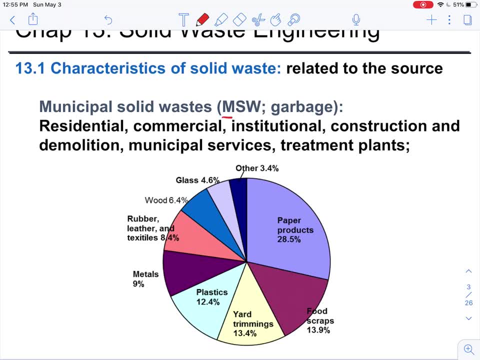 Generating more solid waste. So what is So, what is the characteristics of the solid waste? So here in this class, we're going to mainly focus on the municipal solid waste, or the MSW, So we're going to use this acronym quite often. 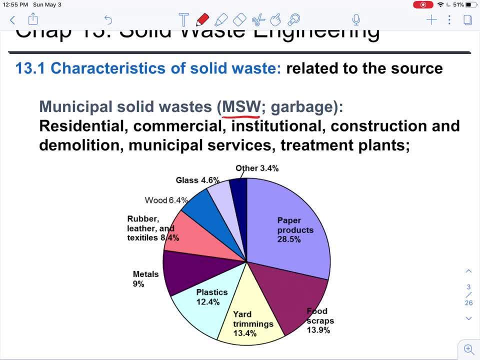 So we also call them as garbage right. So the MSW or the municipal solid waste can come from residential, commercial, institutional construction demolition right. Civil engineering basically generates a lot of waste Coming out of the constructions in there right. 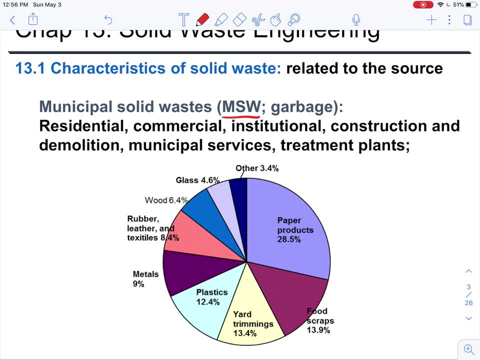 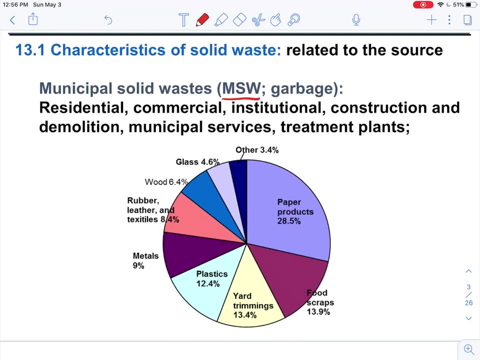 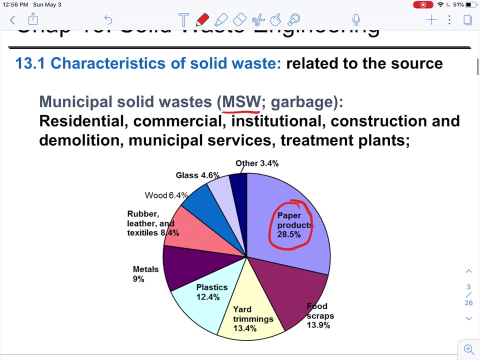 So municipal services, treatment plants, so on and so forth. okay, So if you make a pie chart of all of these solid waste, you can see that a major composition of it are actually paper products. okay, And then we have food scraps, yard trimming plastics, metal, rubber, leather, right. 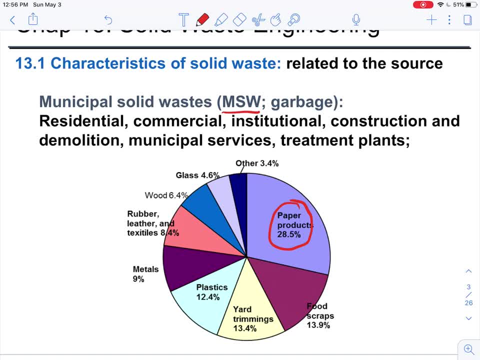 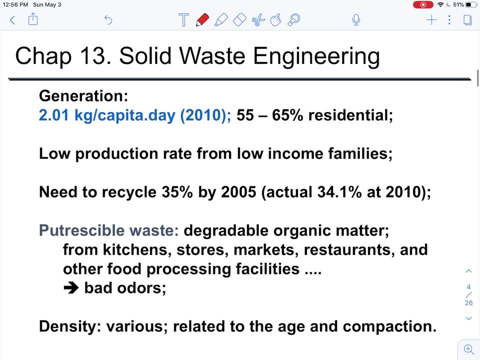 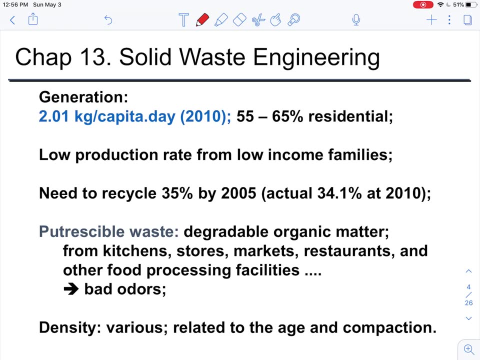 So these generally will occupy a smaller fraction of the pie chart, So Most of them are actually paper And in terms of the generation, so based on statistics of 2010,. so each person basically generate 2.01 kilogram per day. 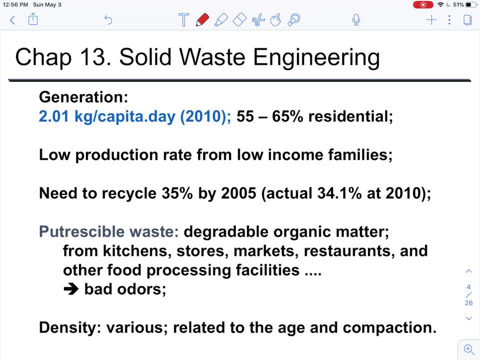 This is not a very significant amount of solid waste, right? So actually 55 to 65% are coming from the residential And there's also low production rate from low income, in fact Income, in fact Families. okay, So basically there was also a plan that people want to recycle: 35 by the year of 2005.. 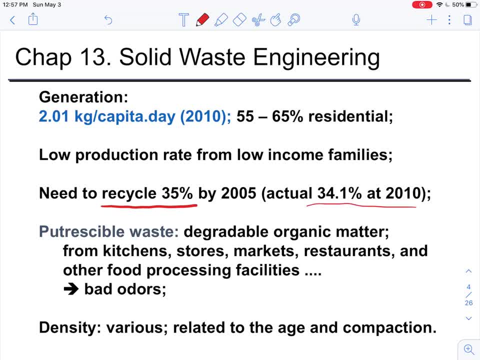 But actually in 2010,, the recycle fraction is 34.1%. Basically, it's a little bit lower than the expectation, okay. So in terms of the solid waste, people also will categorize, or one type of it, It's called the. 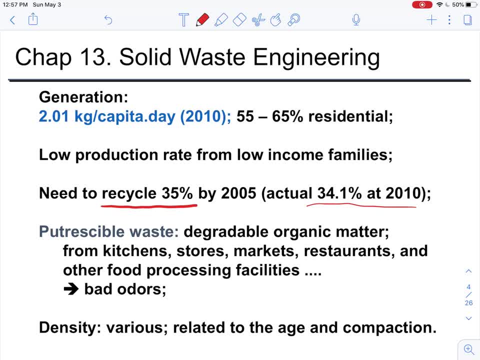 Protractable waste, So, which means that they can degrade. okay, So these degradable organic matter can come from kitchens, stores, markets, restaurants and so on and so forth, But while they're being degraded, they will generate bad odors. 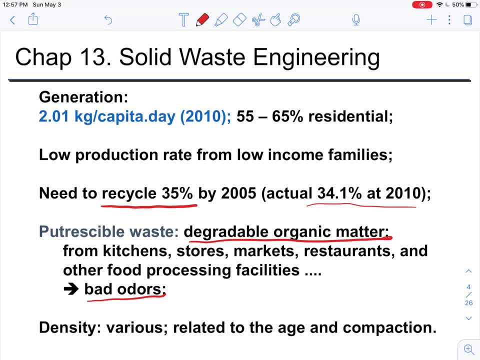 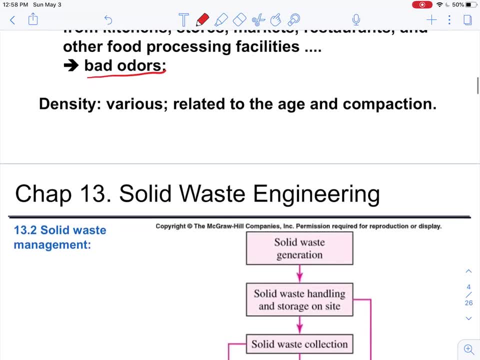 And in terms of density, they can have different types of density or depend Really depends on what type of solid waste we're talking about And also related to the age and compaction. So, in terms of the solid waste we're talking about, 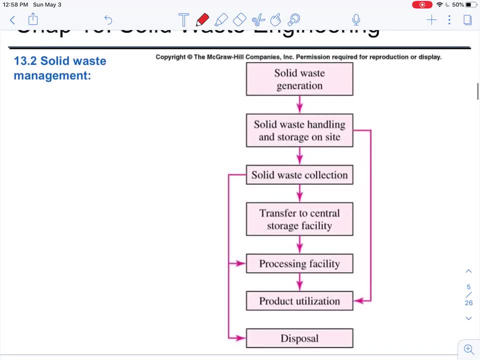 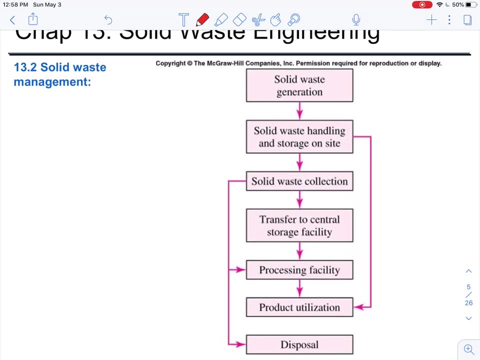 So, in terms of the solid waste we're talking about, So, in terms of the solid waste we're talking about, In terms of the solid waste management, there are several rules, And then I think that this is the diagram that we showed during the first chapter here. 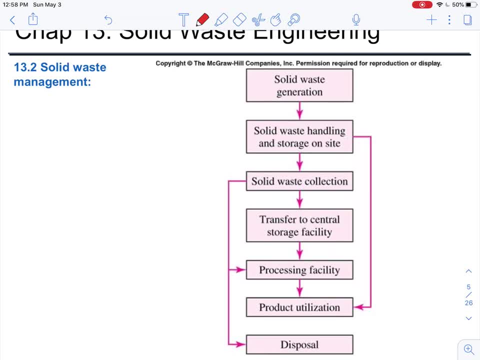 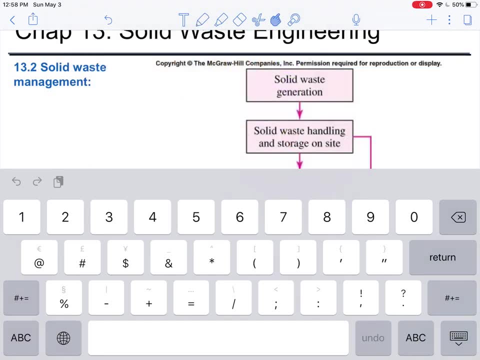 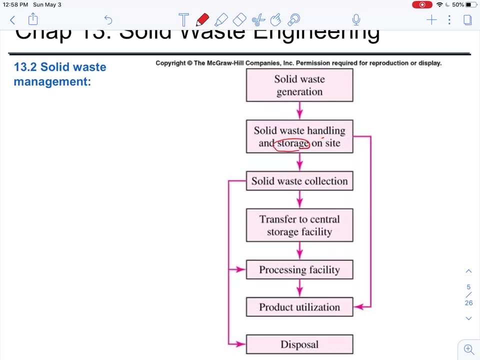 So if we try to track the lifetime of the solid waste, So they're first being generated and then they're being handled- Okay, Let me remove this. So they are being handled on-site and also stored right, And further they can be transported to solid waste collection and then transfer to a storage facility. 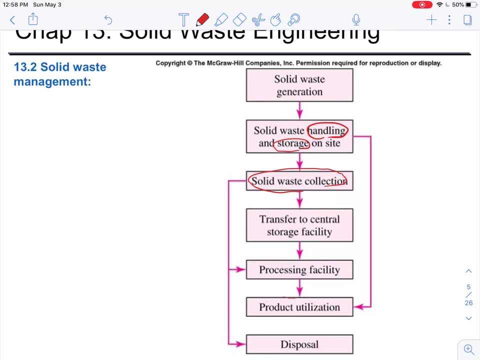 And also some of them can be processed right. Some of them can even get recycled right. So this is product utilization. So if this solid waste handling and storage is already a central facility, then you can directly process all of these wastes and also reutilize right. 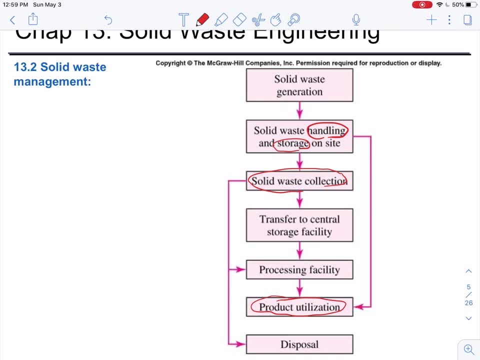 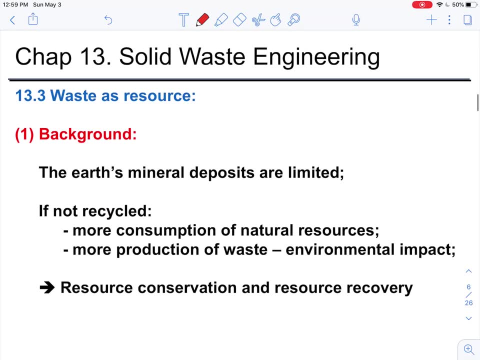 To recycle some of the fractions, But some of them cannot be utilized, so they will directly go to disposal. okay, So actually these solid wastes can act as a resource, So there are more efforts trying to recycle a lot of these solid wastes. 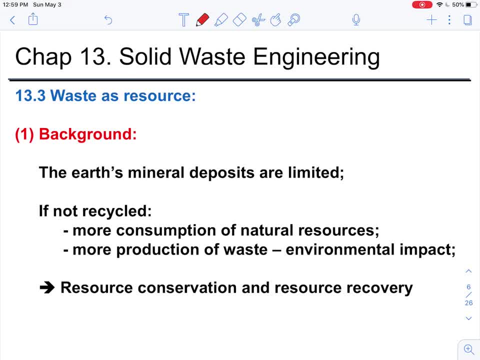 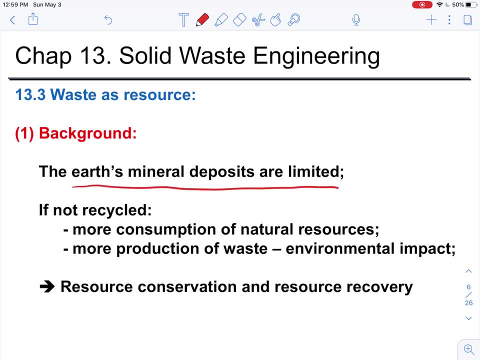 because there are already limited sources, limited resources of the major components in these solid wastes, For example. the earth's mineral deposits are quite limited And if we use more, if we just basically generate more of these mineral deposits, it's going to harm the environment, right. 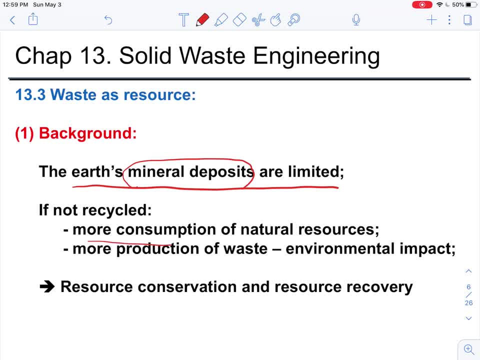 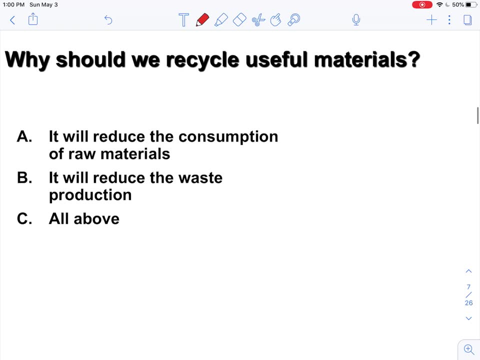 If it's not recycled, the more consumption of the natural resources will happen and also will produce more waste. It's going to cause an environmental impact. So we have to conserve these resources Okay And conduct the recovery of these wastes okay. 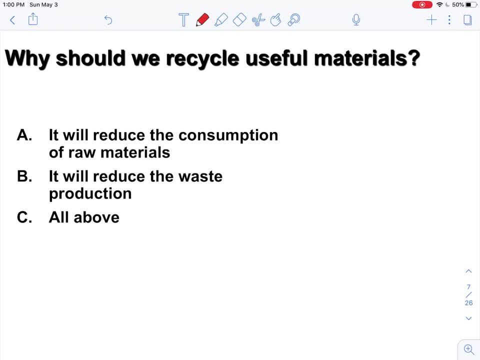 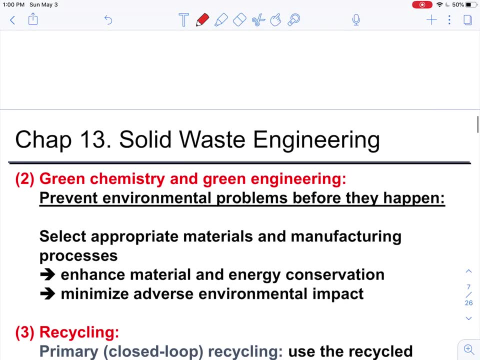 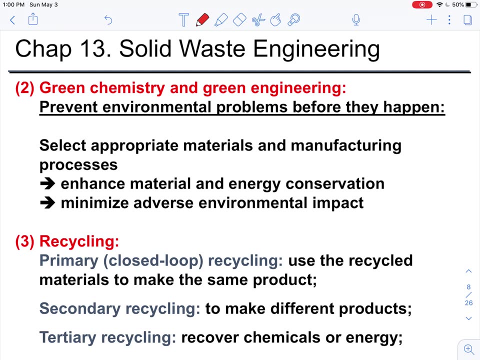 So if you have a question, why should we recycle useful materials? Then we know that it will reduce the consumption and also reduce the waste production. So we'll choose C here, okay, So this idea involves the concept of the green chemistry or the green engineering right. 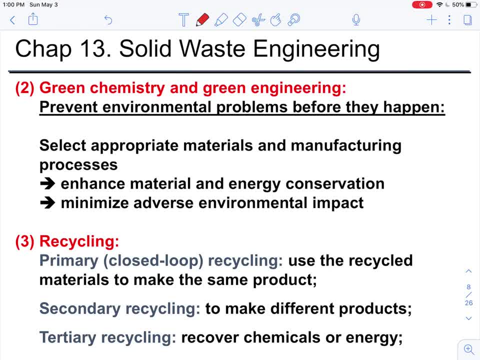 So if you talk about green, then that means more environmental right. So we will try to prevent the environmental problems before they happen, So we can select appropriate materials and manufacturing processes to enhance the material and energy conservation and also to minimize the adverse environmental impact. 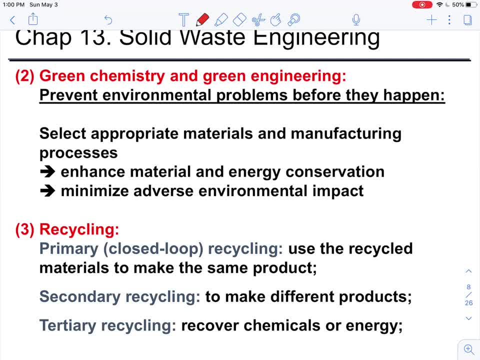 And in terms of the recycling and the modes of the recycling, there can be primary, secondary and tertiary. It really depends on what type of solid waste we're talking about, right? If it's primary recycling, that simply means the recycled material. 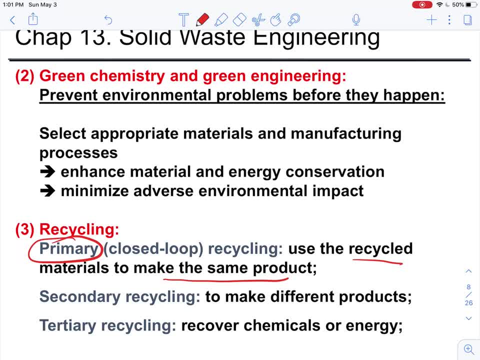 they can be used to form the same product, For example, the plastic bottle that we use coming out of soda bottle, of soda right. So they're made of the same material. they're very stable, they're very endurable, So we can recycle this material after cleaning them. 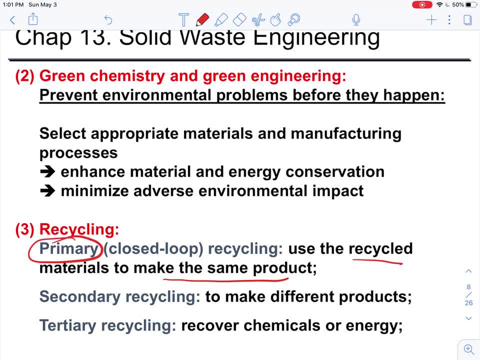 and then manufacture those bottles again. There can be secondary recycling. So basically we can extract some proportion coming out of the solid waste to make different products, For example the electronic waste. We know that there are a lot of noble metals, for example gold, silver, platinum, right. 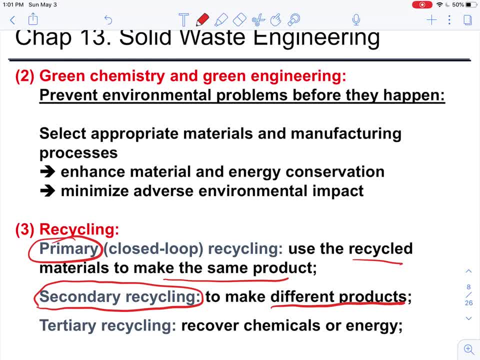 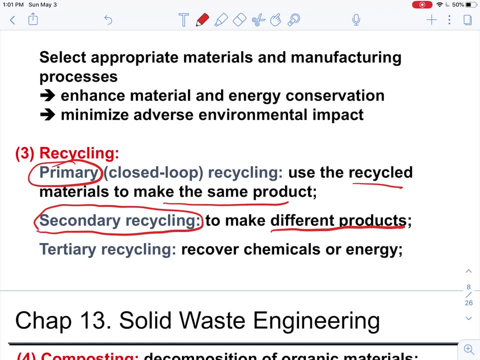 Silicon is not a metal there, but it can also get recycled. So we can extract these metal and other components and make other products right, And there can be tertiary recycling. So tertiary recycling just means to consume them. Basically, one way of consuming them is 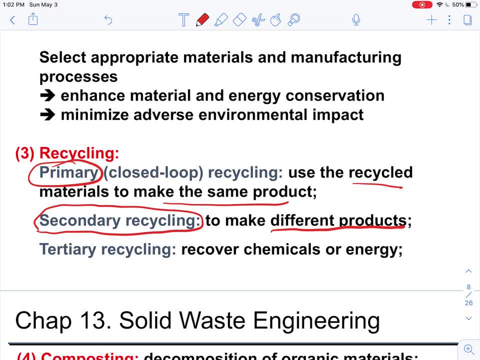 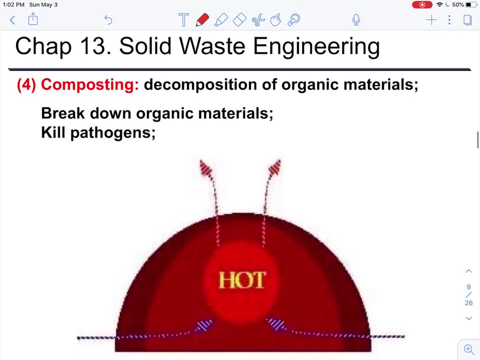 to generate the same amount of material, To generate heat right, Directly burn them and to recover the chemicals and the energy. okay, So that's why, for processing these solid waste, there's an idea called the compositing. So compositing means just to decompose it of these organic materials by using heat. 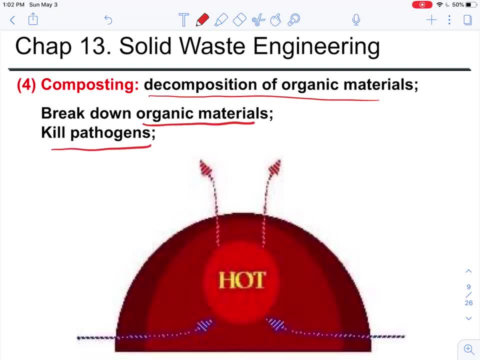 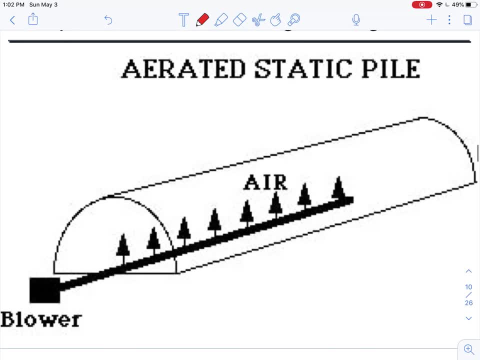 So we break down the organic matters, kill the pathogens and also generate heat where we can utilize this energy. okay, For example, this is a process for the decompositing facility. right, So we have blower that's pumping air inside. 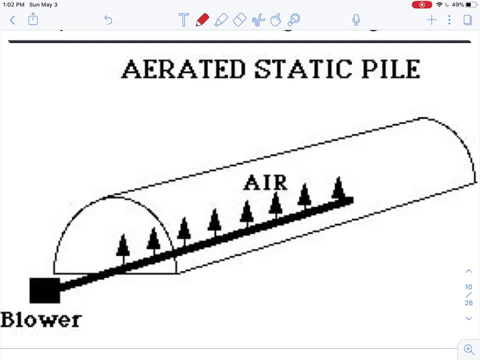 So the air contains oxygen? right, We can decomposite these organic matter to broke them up, because if they're not being decomposited and directly dumped into the atmosphere- and we know that, since they're organic, they're going to increase the BOD of the water resources- okay, 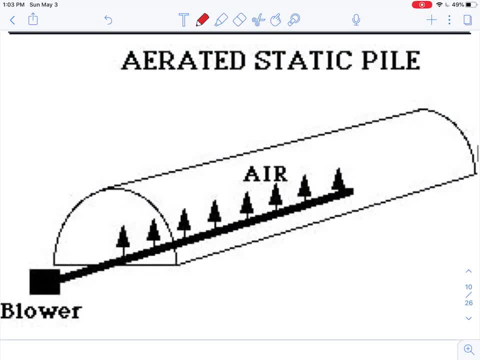 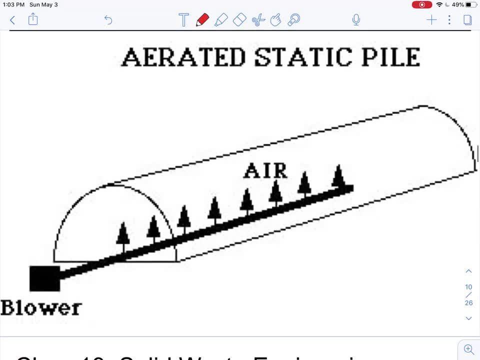 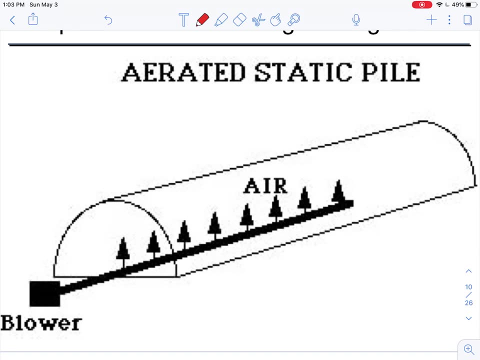 So basically, this process is a batch process. right, So we pump in the air right After the solid waste are decomposed, right, So we take all these products out of this reactor. So the batch reactor. the disadvantage is that we have to transport material in and 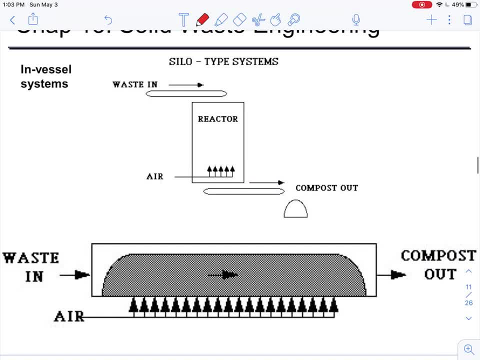 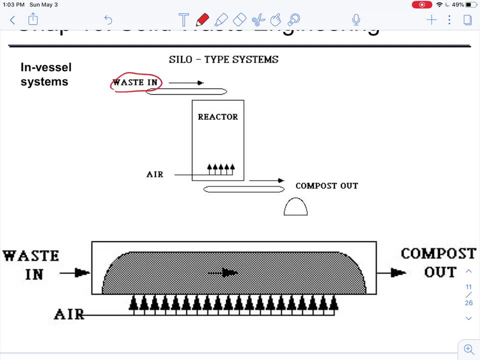 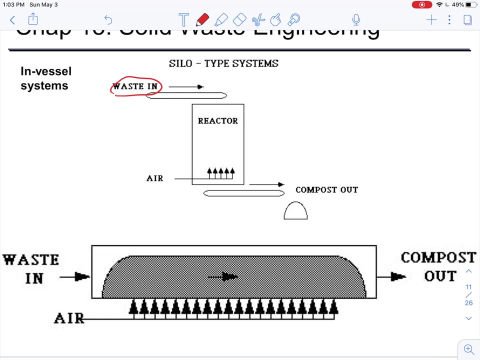 take them out. The reactor have to be stopped. So there's also a continuous process where you use belt to transfer these waste right And also you pump in air right. The product will just also use these belts to transport them out. 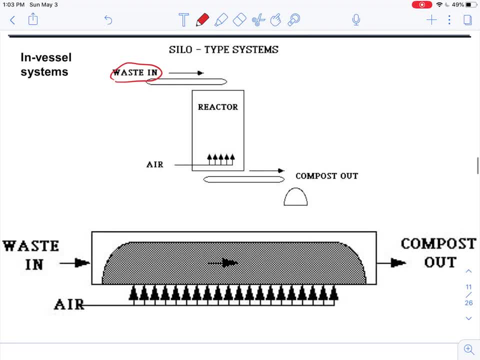 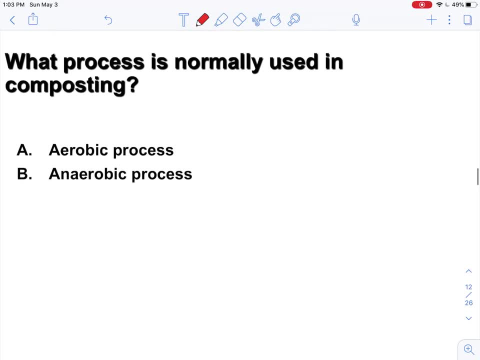 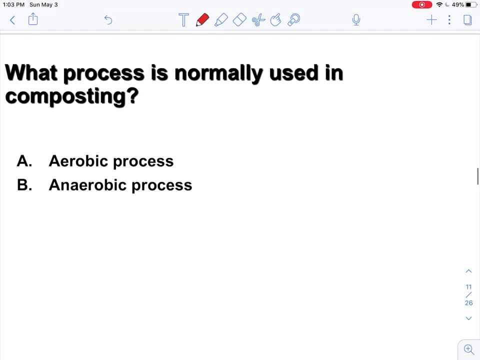 So this is a continuous process And similarly we can use this design here. So this process is also called the in-vessel systems. So here's a question: What process is normally used in decompositing? So, if you think back on the process, what we pump in, what we pump out, what we decompose? 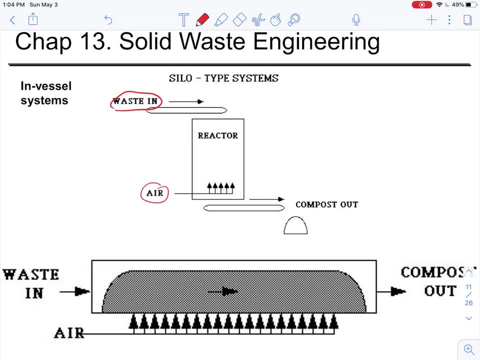 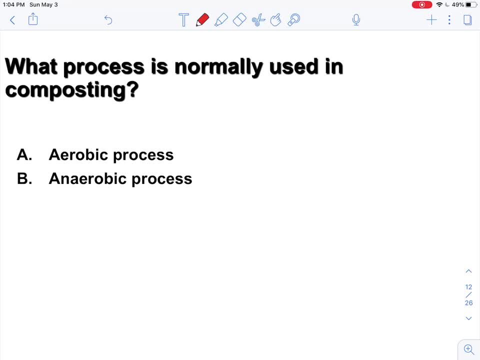 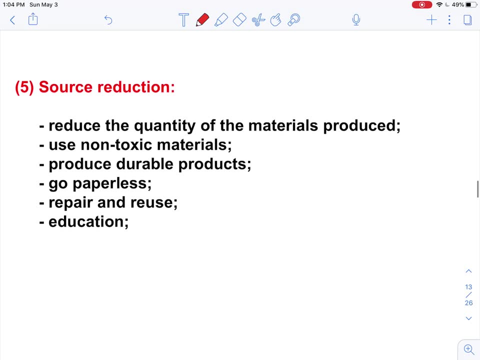 right, We pump in the air, So we're basically using the oxygen in the air to decompose the materials inside, right? So then that's going to be aerobic. It's not anaerobic? okay, Aerobic process. So to alleviate these solid waste problems, we can also reduce the sources. 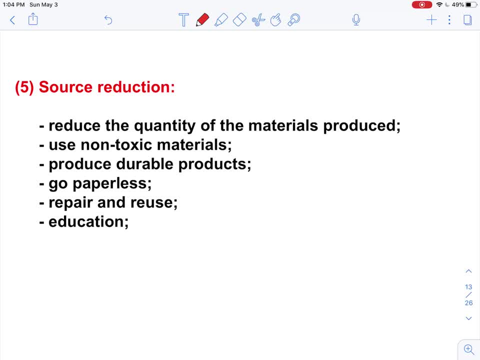 Simply means that we generate less solid waste. okay, So we can conduct the following things: For example, reduce the quantity of the materials produced. use non-toxic materials, So that's going to be more convenient for us to process the solid waste. 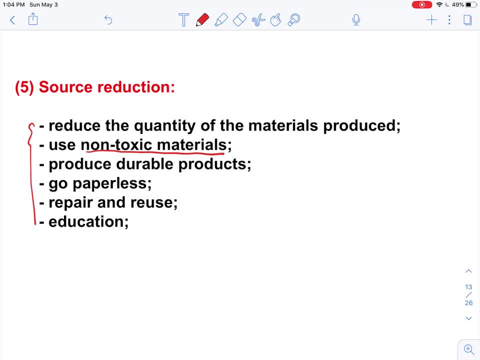 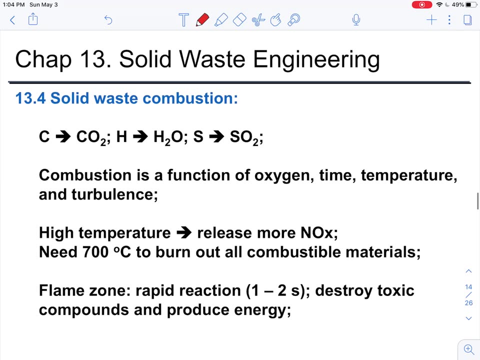 Produce durable products so they degrade less often. We can use them for a very long time. right: Go paperless. If you want to receive bills, you should use electronic bills. right: Repair and reuse education right. So we also mentioned that we can extract the heat. 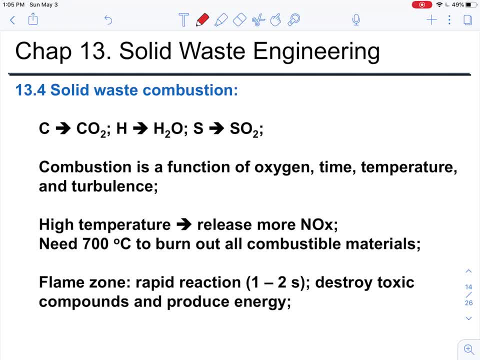 Heat coming out of the solid waste. So that's why people conduct these combustion processes: to downgrade the solid waste. So what it does- tries to do- is convert all of those carbon to carbon dioxide, hydrogen to water and then sulfur to sulfur dioxide. similarly for other types of organics. 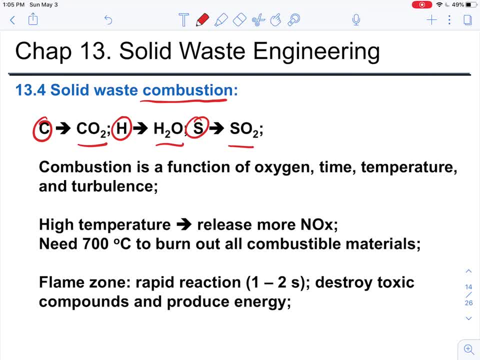 We basically oxidize all of them, generate heat and then potentially generate electricity. So, as we learned From the NOx control, we know that the higher the temperature, the more the NOx is going to form, going to be formed right. 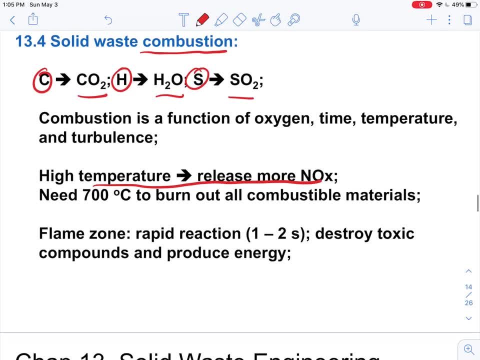 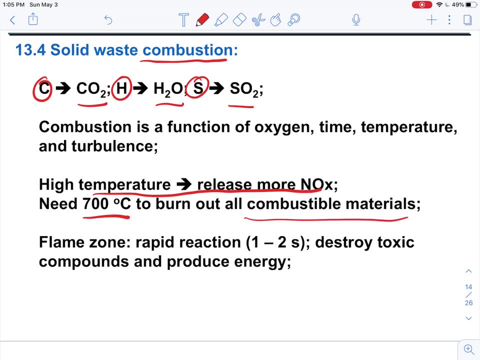 So, basically, this high temperature is going to release more NOx, right, So we need to use 700 Celsius, at least 700 Celsius, to burn out all the combustible materials, But if the temperature is higher, then there will be no more NOx. 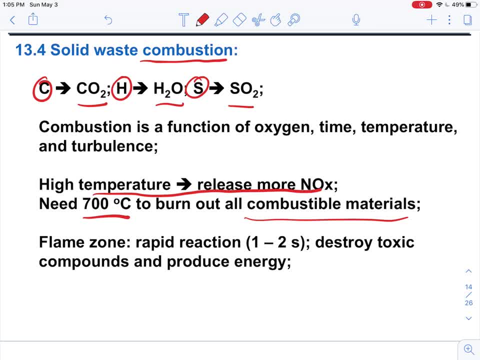 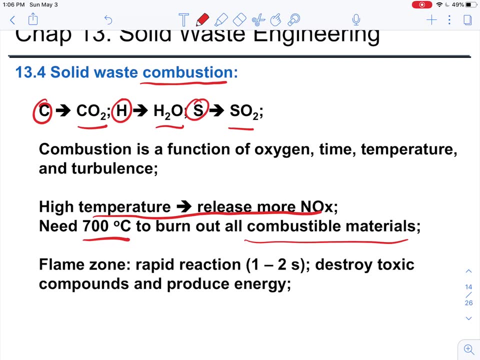 So this process that burns all of these solid waste have to go through the air pollution control. right So we need to use proper devices to remove these air pollutants. right So in the flame zone, typically for these incineration process, there is going to be. 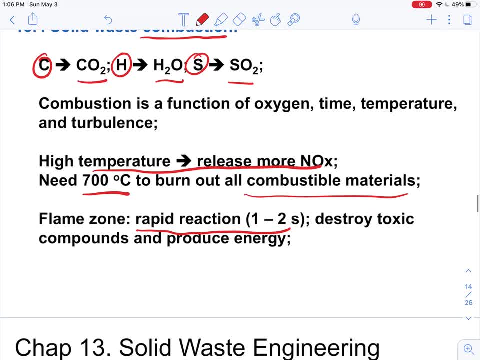 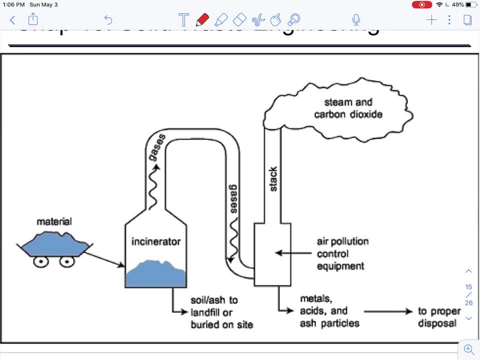 a rapid reaction in one to two seconds to destroy these toxic compounds and produce the energy. So this is, then, a diagram of this solid waste incinerator, So you can see that, after we introduce these solid waste right Inside the incinerator, 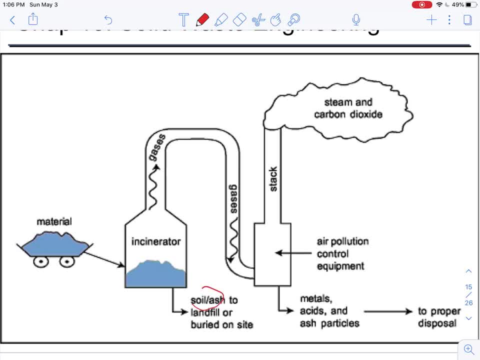 It's getting combusted, We can form the soil or ash coming out of the combustion And these gases are going through these air pollution control equipment right, And then basically, finally, we're going to generate carbon dioxide and water, But there will also be some air pollutants, because we know that the efficient of these 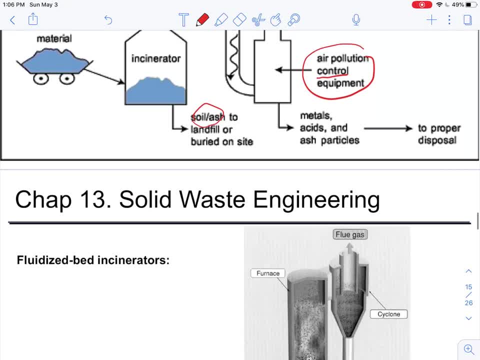 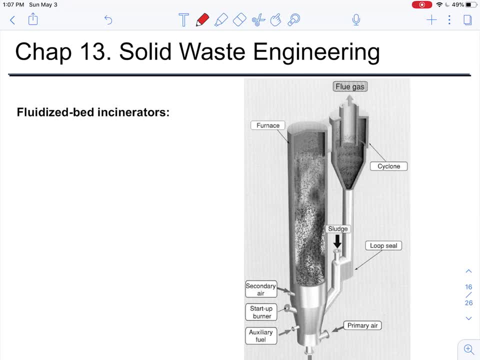 air pollution control equipment is not 100 percent okay. So people also designed Okay These fluidized bed incinerators where the solid waste can be just resuspended in the reactor. So there's more: there's a longer residence time of these reactants in the air. 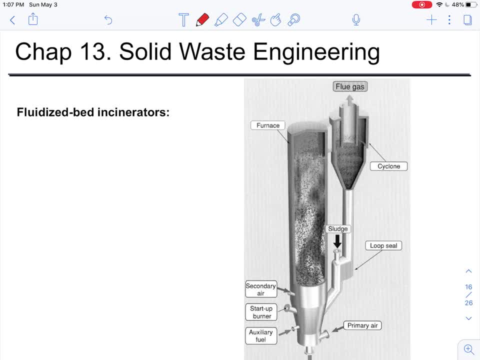 So basically, we generate them, suspended these in small particles and pumping a lot of air, So it's just like bubbling air through solids. So they can be suspended in this vessel here And then, once they are getting combusted, Some of these solids can. 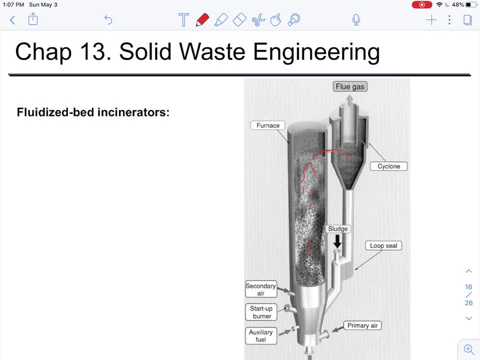 Be pumped into the flue gas And then here we have a cyclone. We know that the cyclone will remove these particulates and then they can settle down and then come back to the reactor. So by recycling them in this fluidized bed reactor we can elongate the residence time. 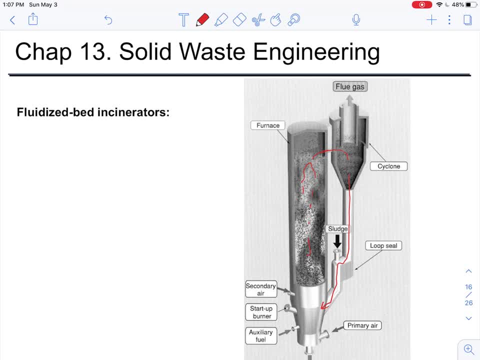 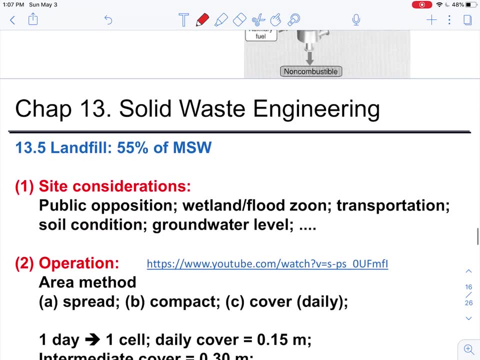 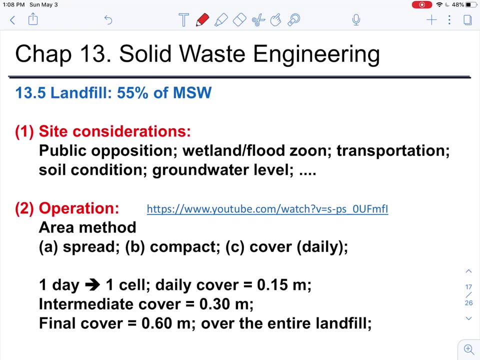 of these solid waste and then try to extract more energy coming out of it and also conduct more complete combustion from these solid waste. Okay, Okay. So the question is one form of the of processing these solid waste. So actually, more than half of these municipal solid waste are directly dumped through landfills. 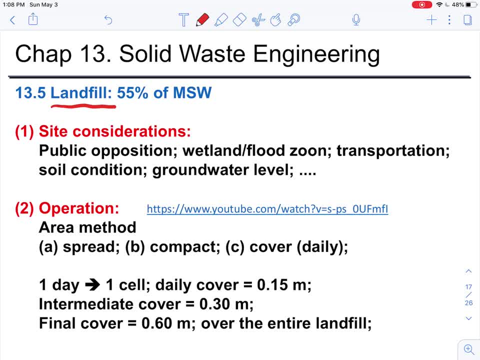 Okay. So if you can, if you want to design a land field, of course you have to think a lot of think about a lot of factors there. You cannot directly decide to build land field nearby your house, Right? So that's not land field, that's littering. 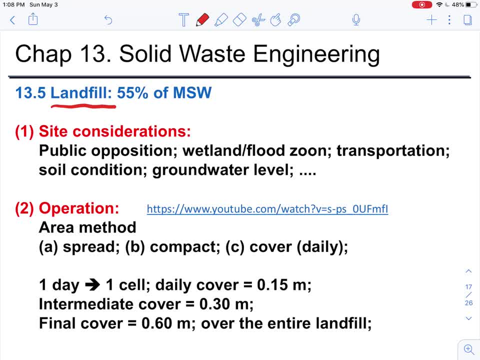 Okay, So in terms of these large land fields, there are a lot of site considerations. For example, people need to think about the public opposition. No one wants to build a land field beside their homes, right, And people need to talk, need to think about the wetland or flood zone, because a lot of 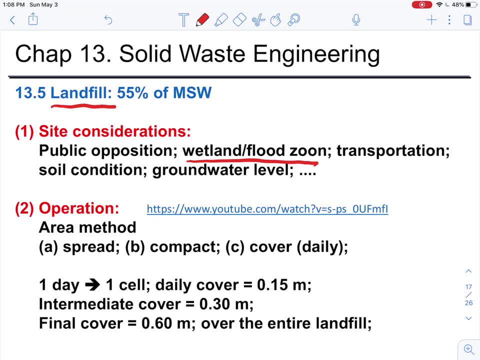 water. if they get through these solid waste, there might be some wasted or polluted liquids. right, There's a specific name for those waste liquid or polluted liquid there. We're going to talk about that later. And people also need to think about the transportation. 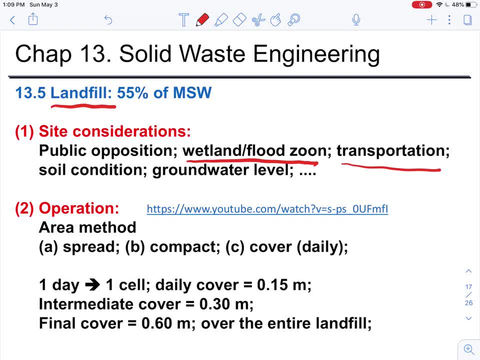 You can't really build a land field. that's really far away. Of course people want to make these, build these land fields as far away as possible, but we need to consider about the transportation, We need to think about the soil condition because once we form those polluted liquid, 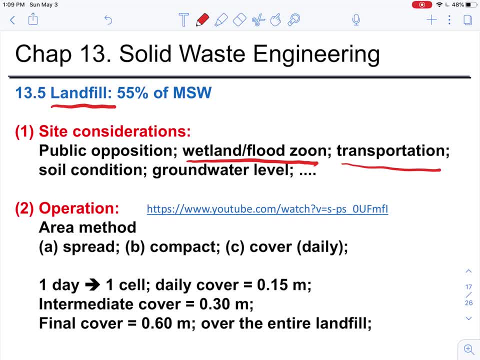 they can be transported in soil, And then we want a smaller velocity of these pollutants in the soil because they might get permeated through the drinkable water, underground water and polluted water resources. Also, we need to consider about the groundwater level. Okay, 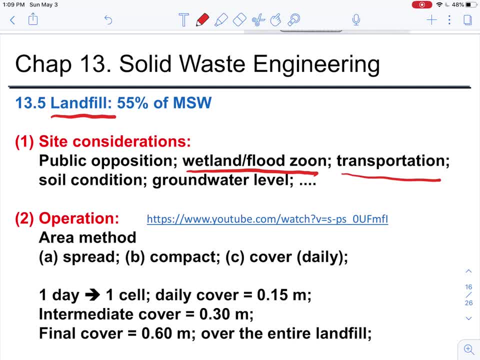 So in terms of the operation of these land field, there are basically three steps right. First we'll spread them to basically remove, Or remove some easily degradable components there, and then we'll compact, So basically form a more compact structure, and then we'll pack them in the land field. 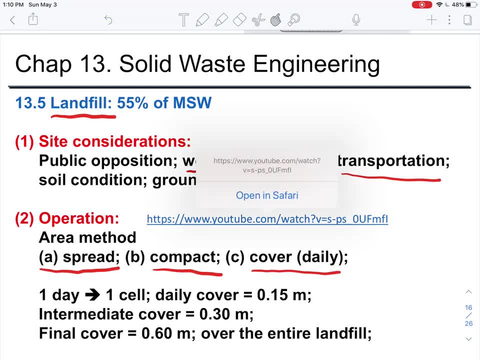 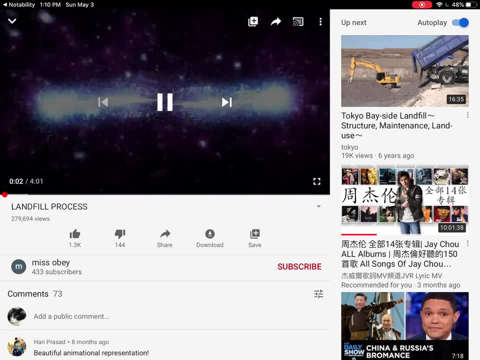 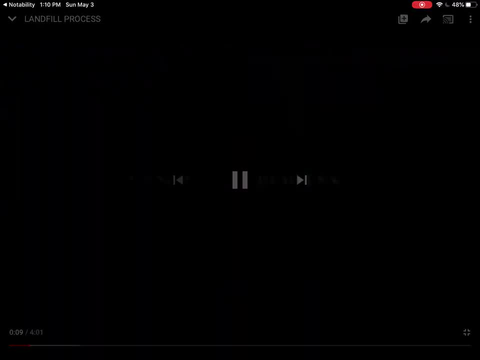 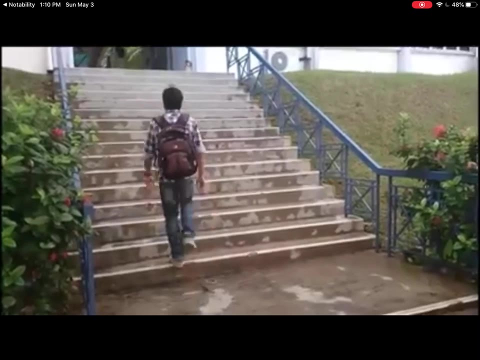 Okay, So here I have a short video regarding the operation of the land field, So let's try to watch through them And we can start by removing the original system. Skip a little bit. 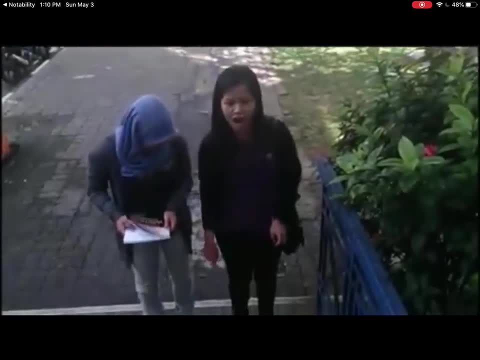 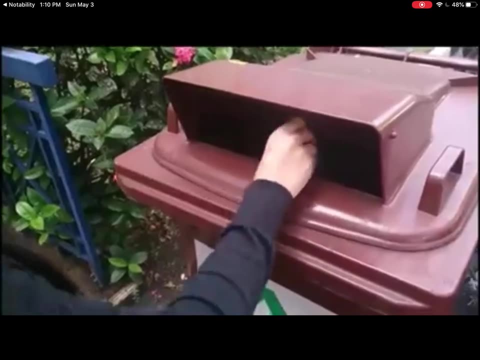 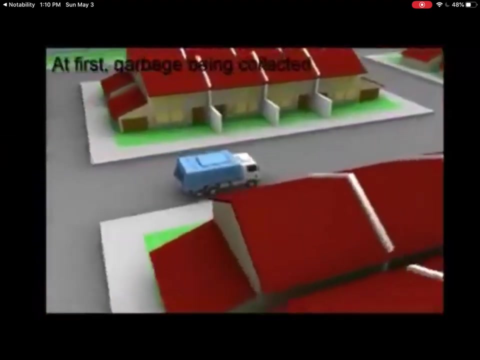 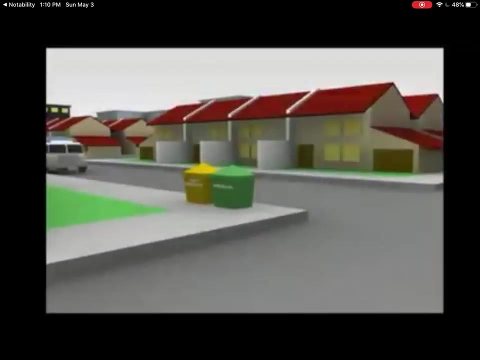 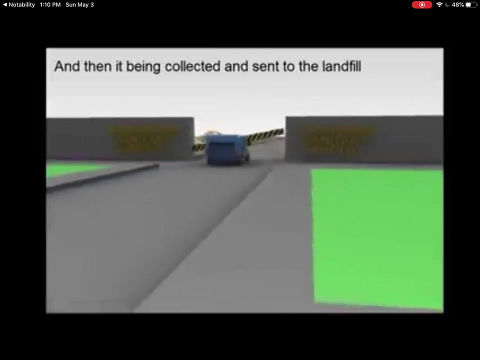 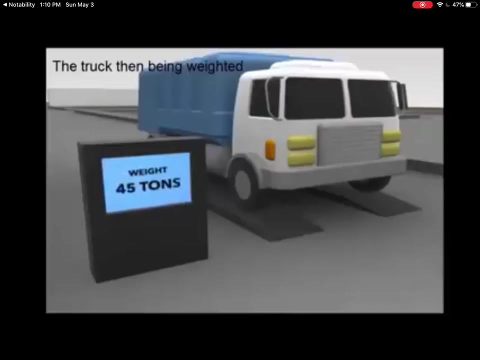 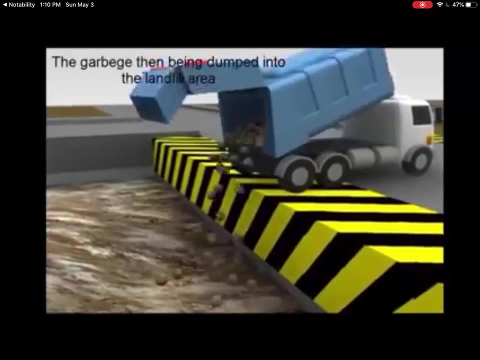 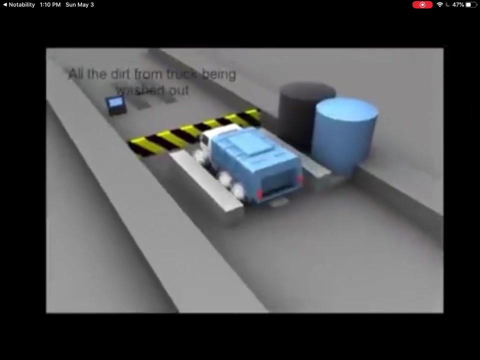 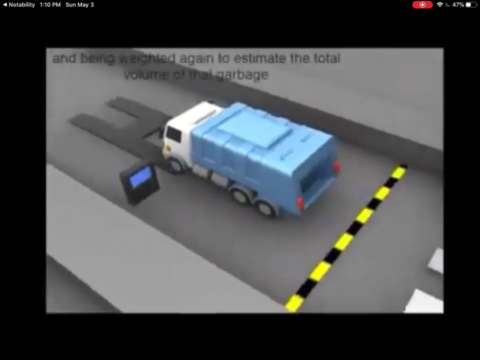 We'll be right back. So basically, after they're collected, we'll spread them to a specific area to basically let the air to go through right to oxidize some easily degradable solutions. 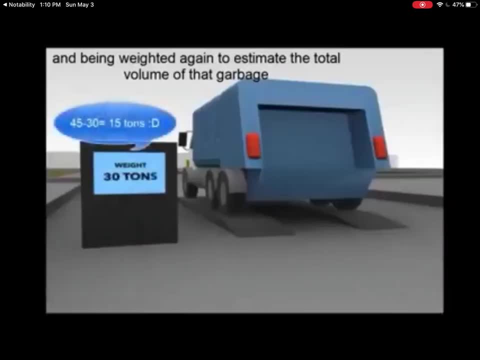 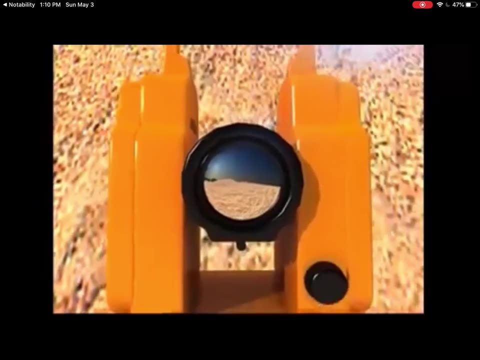 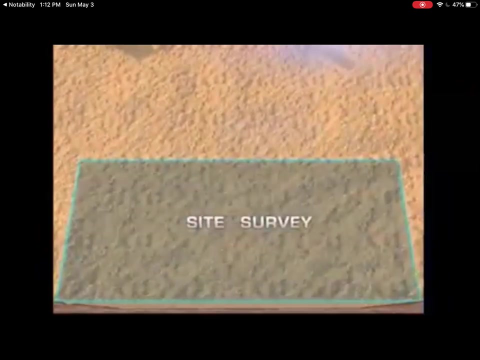 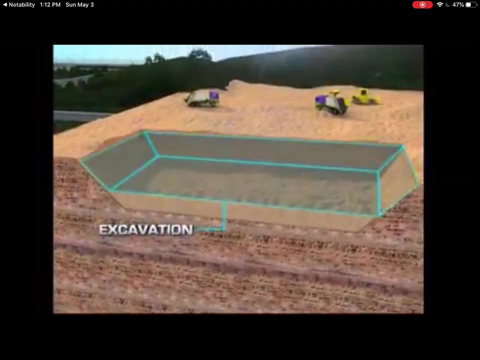 So we'll weigh these trucks to get an idea of how much solid waste we're collecting every year. So this is the actual landfill we're talking about. So people do these site surveys to know what is the soil structure, what is the soil condition there. 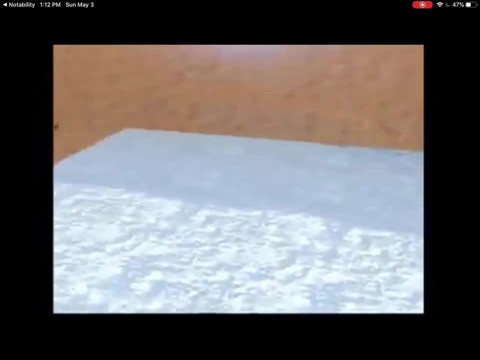 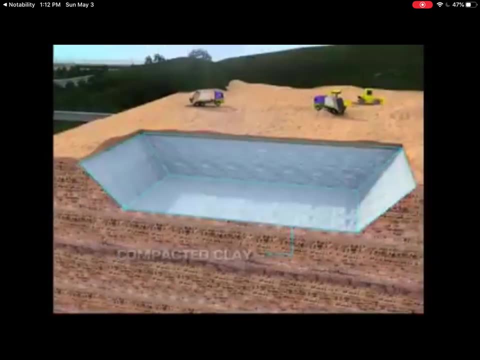 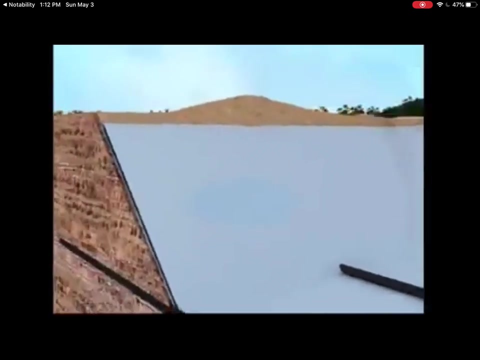 And each of this unit here is called a cell. So what this is doing is basically form a layer, so that we said that there will be coated liquid, right? so we don't let this liquid further permeate through the air, So the soil will pollute the underground water. 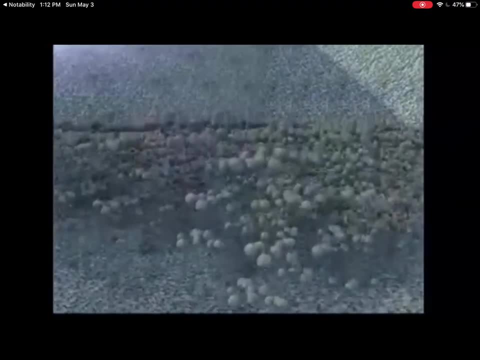 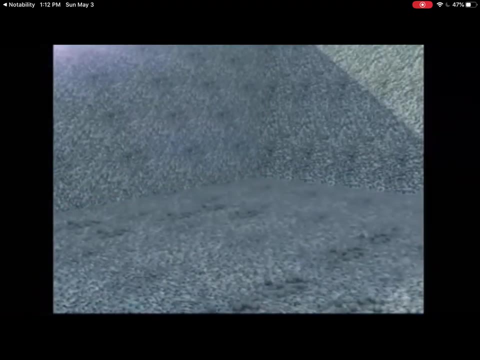 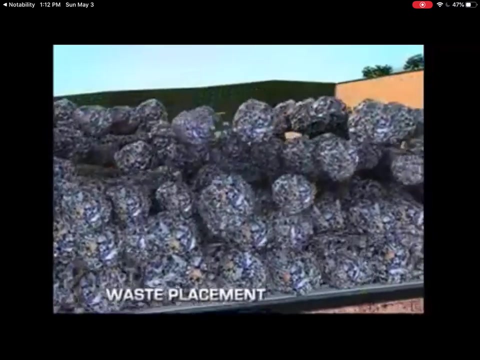 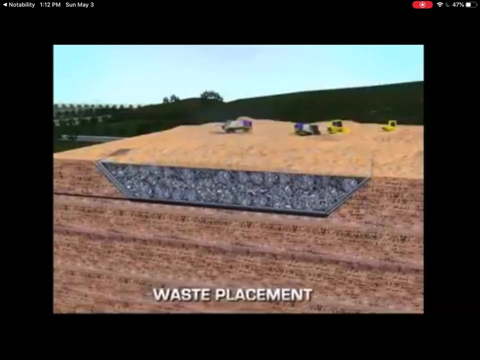 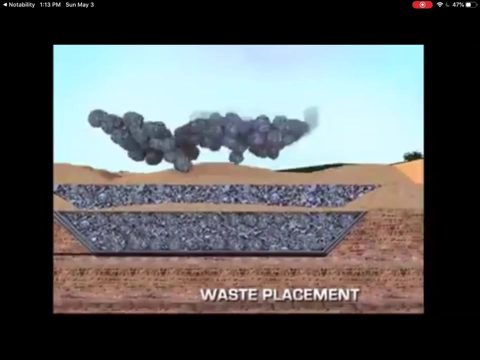 So this coated liquid is called the leachate. So we'll form several layers of these structures here to really stop the penetration of this coated liquid. here for the leachate, This is placing the compacted solid waste And we'll form this daily cover, which is a thin cover of soil above this solid waste. 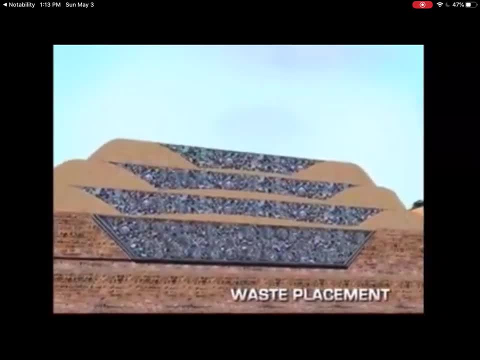 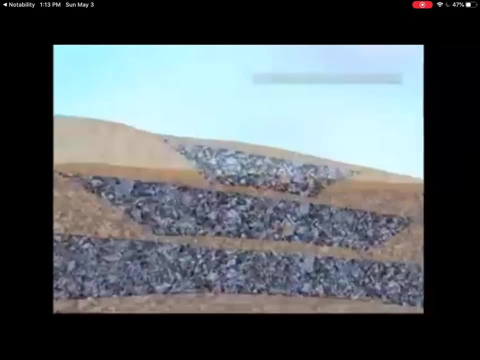 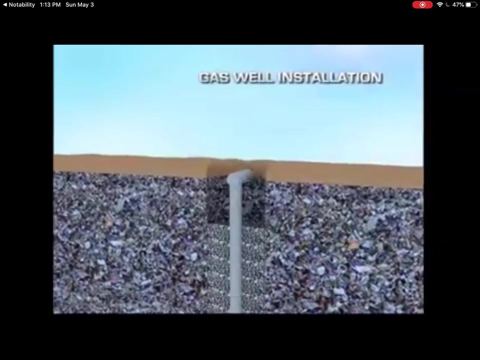 And we can put several cells above it. So finally we have this final cover, which is a solid layer above that, And typically this final cover is thicker compared to the daily cover. So this is using a gas valve. Well, because 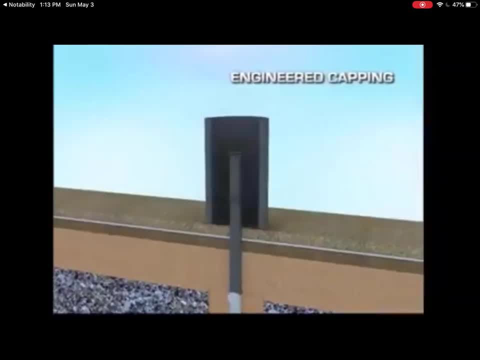 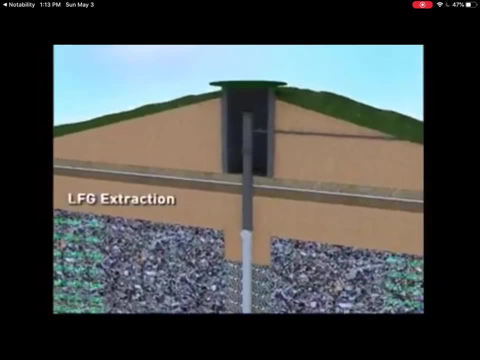 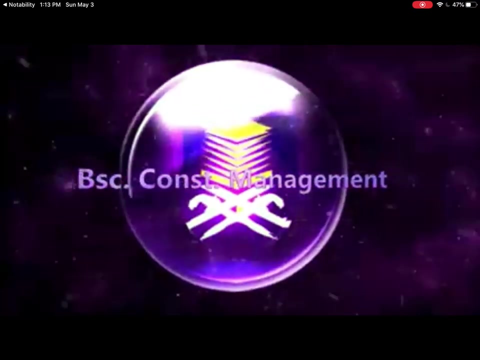 We know that the oxidation of this solid waste or the anaerobic process generates a lot of gas species. So we don't want explosion to happen, right? So we have this valve to transport these gas species or extract these gas species. Okay, so that's it. 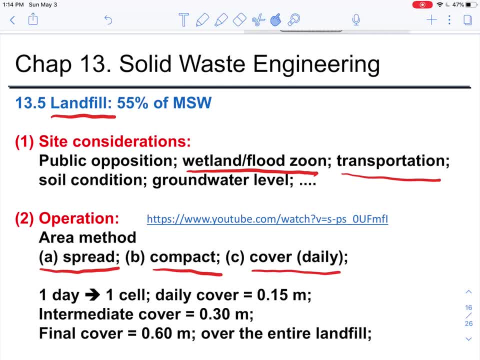 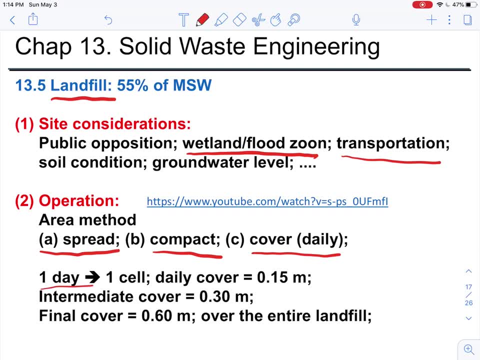 So we can see that there are several processes involved. So we can use it each day for one cell. Of course it depends on how much solid waste we're processing, But we don't want to form these cells several days there, Because once it's exposed to the air for a longer time, then we may generate a lot of air pollutants. 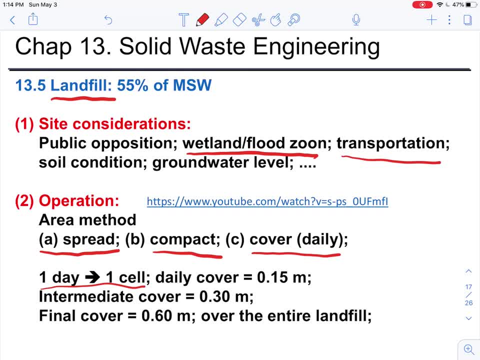 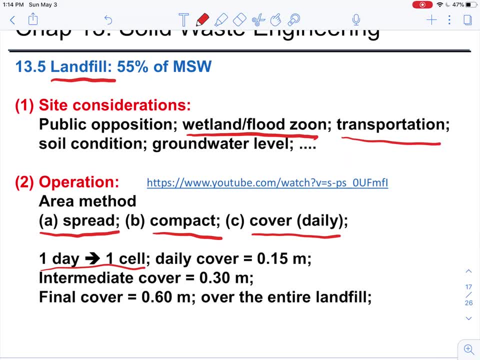 So the daily cover is typically around Okay, 0.15 meter. You can see that this is a relatively thin layer of soil. We also can have intermediate cover, which can happen above several layers of cell, And the final cover has to be thicker simply because we want to prevent these pollutant species to permeate through the top cover and then generate air pollution issues. 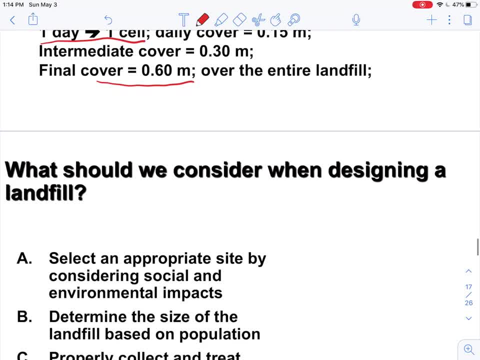 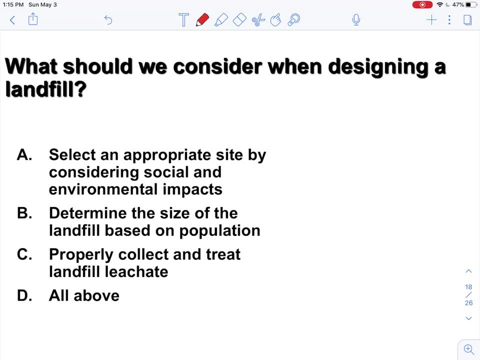 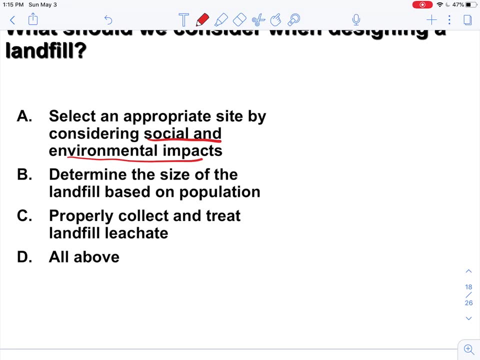 And the final cover is over the entire landfill Landfill. So, again regarding site consideration, what should we consider when we design a landfill right? So we need to consider both the social and environmental impacts, determine the size and length of the landfill based on population, and properly collect and treat these landfill leachate. 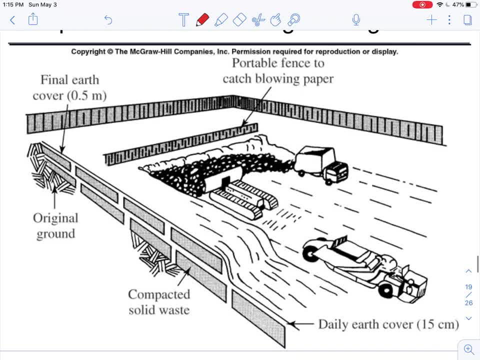 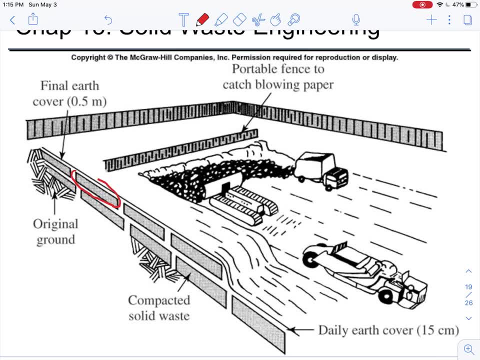 So all of them should be considered. So this is a diagram showing how we process these solid waste here. So basically, you can see that each cell will finally look like this. Of course, this is using. This is using a different structure or different type of structure for processing these solid waste. 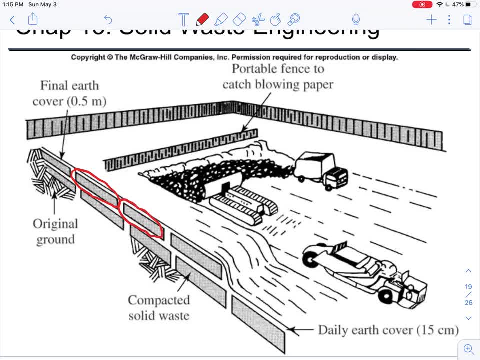 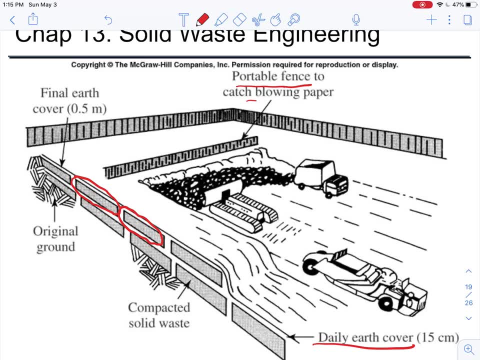 But still we're forming these daily cell here and then covering them by the daily cover, Okay, And also you can see that we have these portable fans to catch the blowing paper, because we know that paper can easily get dispersed in the air. 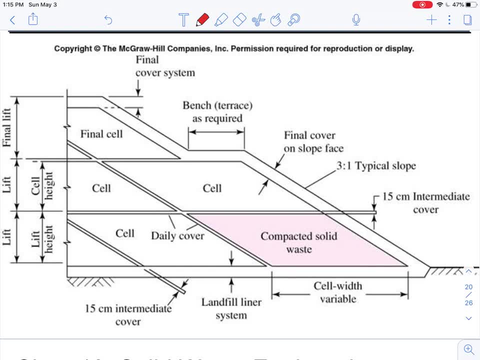 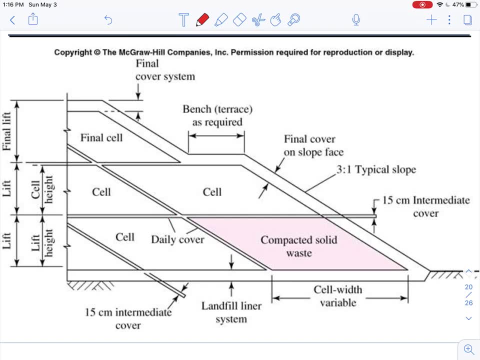 Right. So this is a side view of this landfill. So again you can see these different cells. right between them are the daily cover, right? So inside each cell there are compacted solid waste. So that's after the compaction. 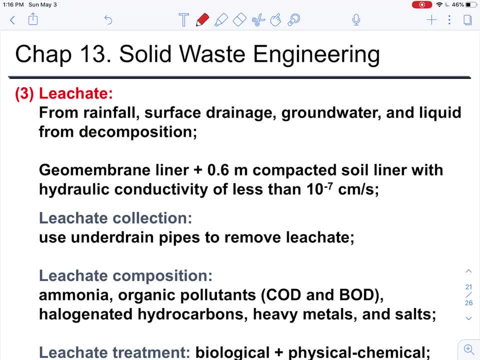 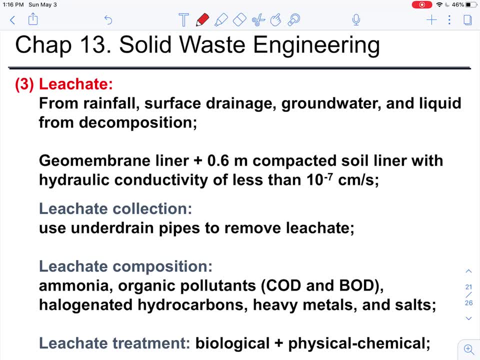 Okay, So we introduced that those polluted liquid are called the leachate. So if you think about the composition of these leachate, they're basically very concentrated polluted waste stream, right Waste stream there. So they can either come from: 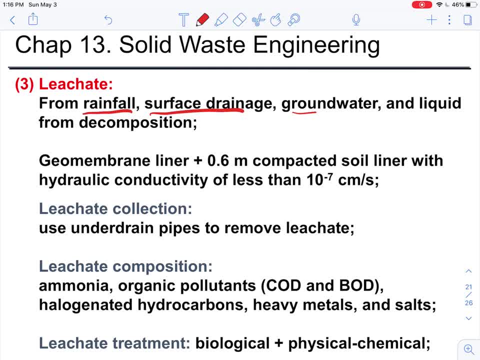 They can come from the rainfall or the surface drainage right, come from the groundwater and also the liquid coming out of the decomposition, and they can be very contain a lot of unpleasant odor there right. So what people do is they'll form these geomembrane liner, which are basically the layer at the bottom of each cell there. 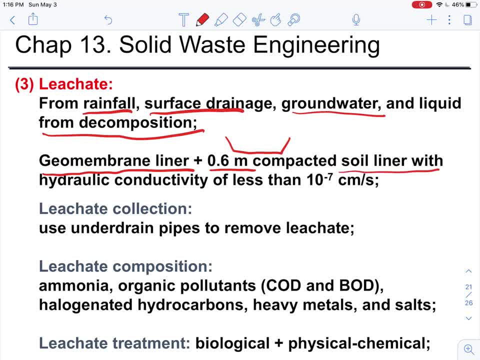 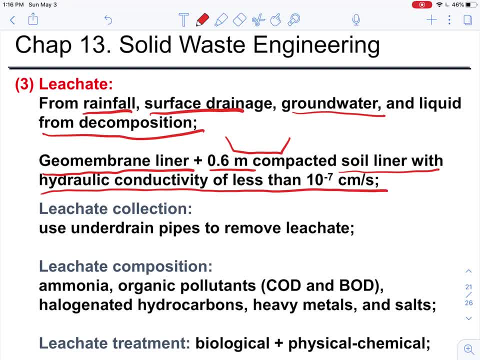 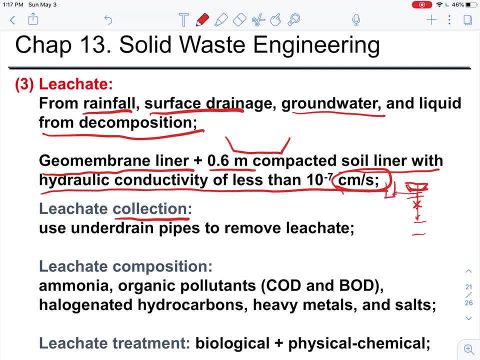 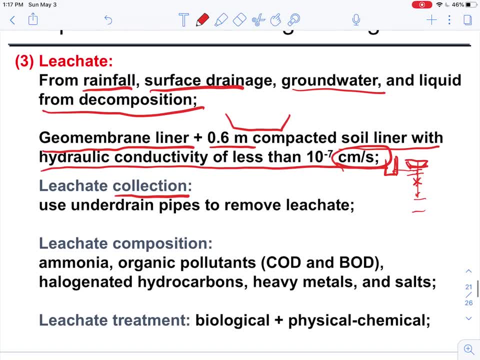 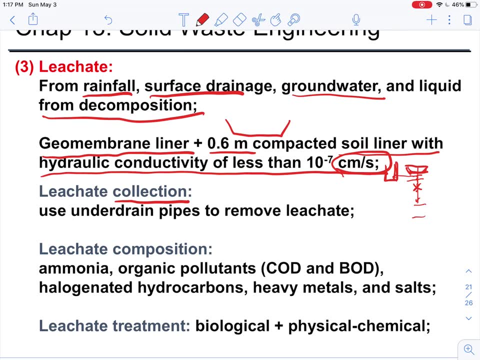 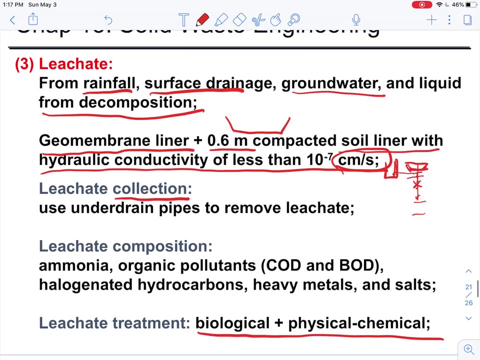 there are pipes to collect these liquid and transfer them into a side. well, here, to collect these liquid, and in terms of the composition or the removal of these, these leachate people can use basically the oxidation process. you can use the biological or physical and chemical method. right, if you think about the composition, they can contain a lot of ammonia, right, organic. 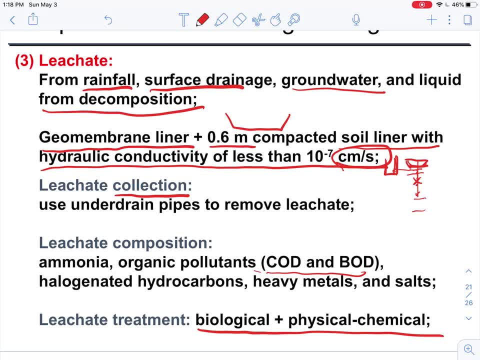 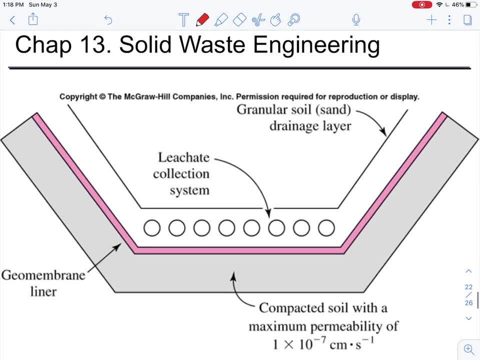 pollutants, which can be both cod and bod, halogenated hydrocarbons, right, heavy metals and salts. okay, so this is another side view of this cell here. so basically we will form these geomembrane here to um or the geomembrane here to prevent the leachate from going through. 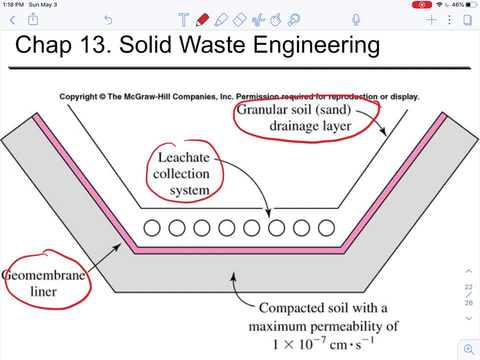 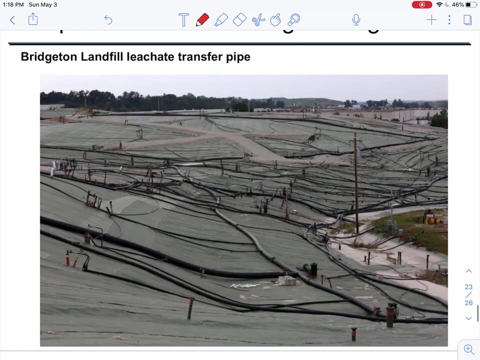 right, we also put in these pipes here to collect these leachate, to centralize them through the, through the wells that's at the site or beside these, beside these cells, okay, so this is a picture showing these leachate transfer pipes. so, finally, the landfill will. 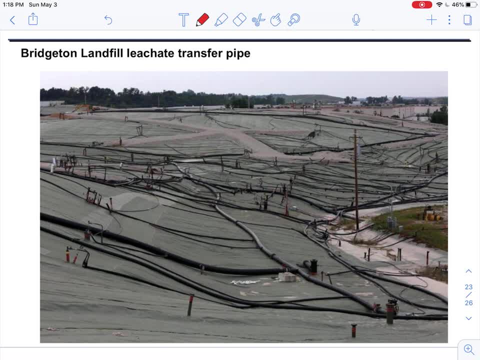 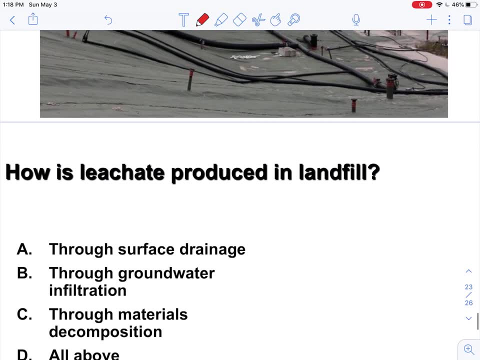 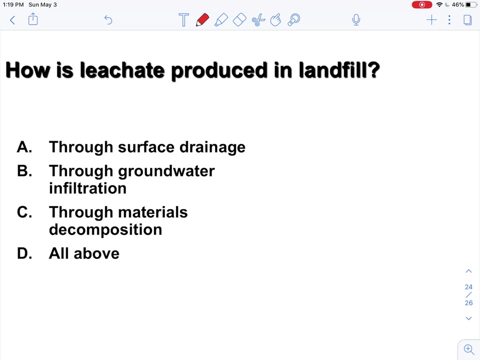 cover all of these pipes, right, but people are building up these pipes in advance because, finally, they're going to process the waste through these facilities. so, if you ask the question, how is leachate being produced in the landfill, or why they are being produced? so they can be produced through the surface drainage right coming from the storm. 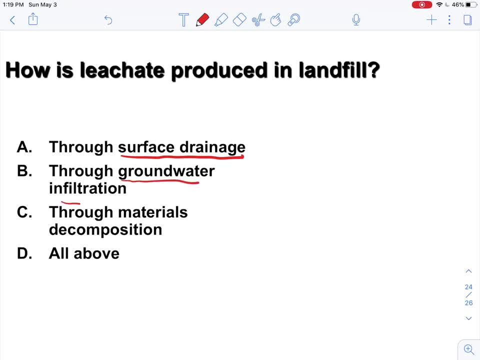 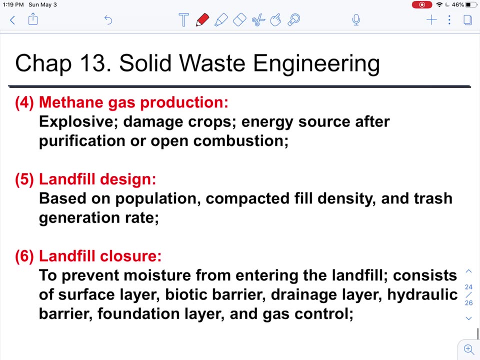 water, rainwater. they can be generated through the groundwater infiltration, so groundwater can also mix, mix up into these cells here, so they can also be generated from the material decomposition. so all, all of them can generate these digits. okay, So in terms of the landfills, 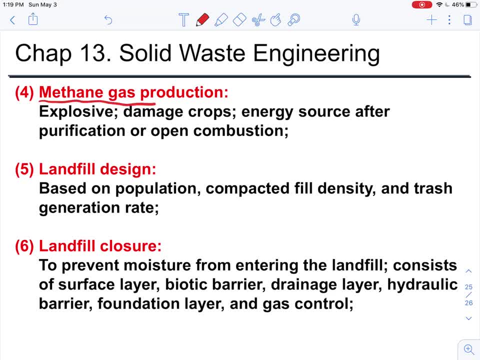 they're also generating methane gas right Coming from the anaerobic processes, because we know the anaerobic process generate these gaseous organics right. So they are hazardous materials because they can easily cause explosion. right, They can damage crops.